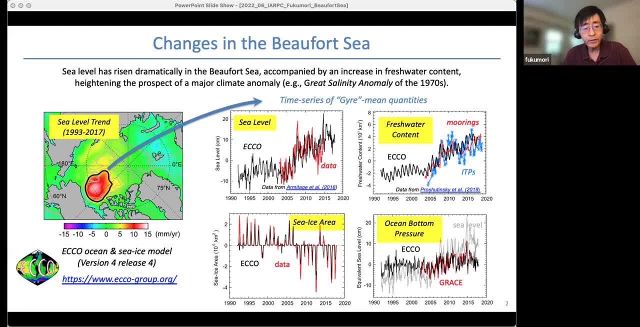 These are anomalies from 1993 to 2017 of quantities averaged within the Beaufort-Jaya region, contoured in black in the left panel, where the ECHO's sea level trend exceeds six millimeters per year over this period relative to its global mean. As many of you are aware, sea level in the Beaufort 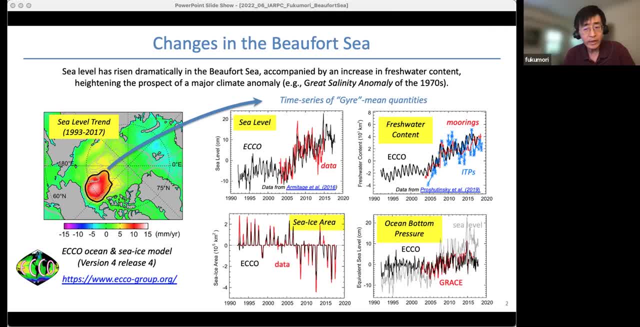 Sea has been rising rapidly during the last two decades, especially after 2007,, shown in the top left, accompanied by an increase in the region's fresh water content. shown in top right. The variations of the ECHO estimate in black are largely consistent with satellite sea level. 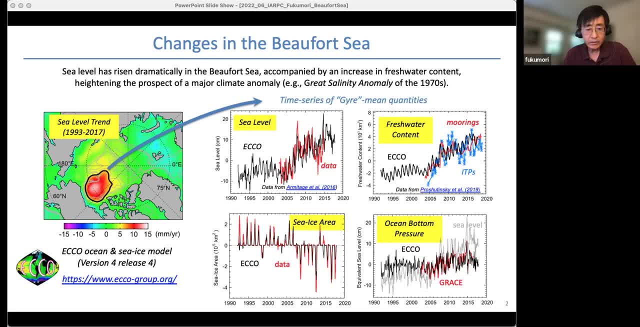 and in situ fresh water content observations analyzed in previous studies. The bottom figures, which also demonstrate consistency between model and data, show sea ice on the left decreasing in the Beaufort Sea also from around 2007, and ocean bottom pressure, plotted to its right, varying at high frequency. 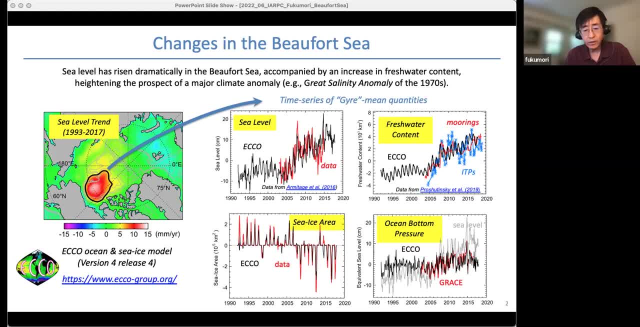 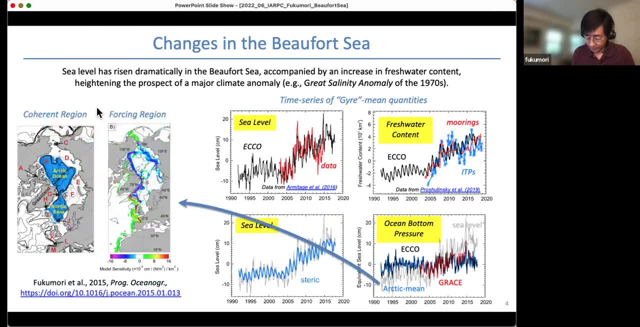 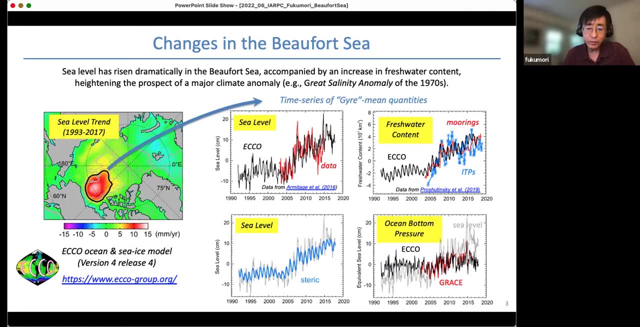 but lacking significant decadal change that's seen in other quantities. The bottom pressure variations, however, explain most of the sea levels: high frequency fluctuation, evidenced by the slowly varying steric sea level shown in blue in the bottom left of this slide. 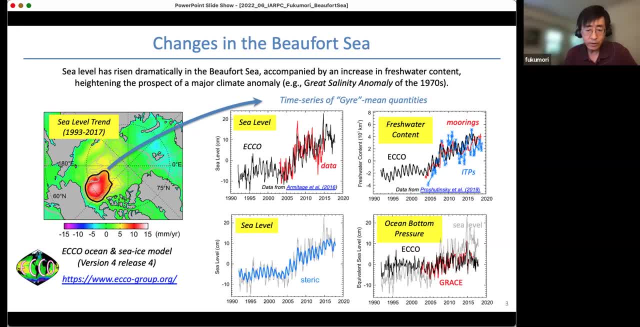 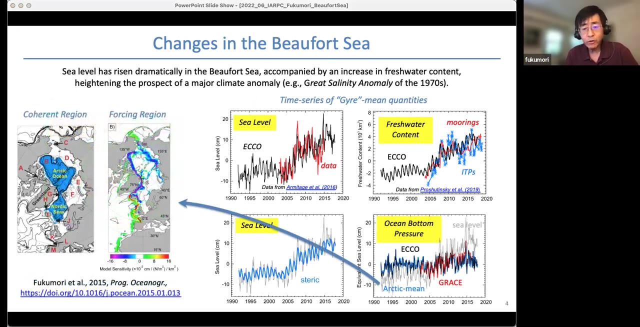 obtained by removing bottom pressure signals from sea level. This blue steric sea level change is almost entirely halo steric, as evidenced by its similarity to the model's freshwater content plotted in the top right. So Beaufort Sea's ocean bottom pressure reflects a near uniform. 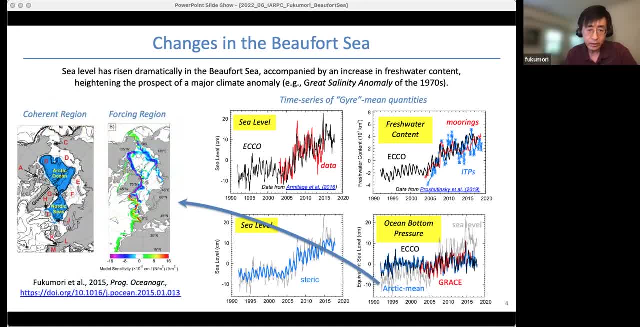 barotropic oscillation that spans a much larger area of the Arctic, as well as the the Nordic seas, whose mean is shown in blue in the time series in the bottom right. that's practically identical to Beaufort Sea's change in black. This pan-Arctic variation was the subject. 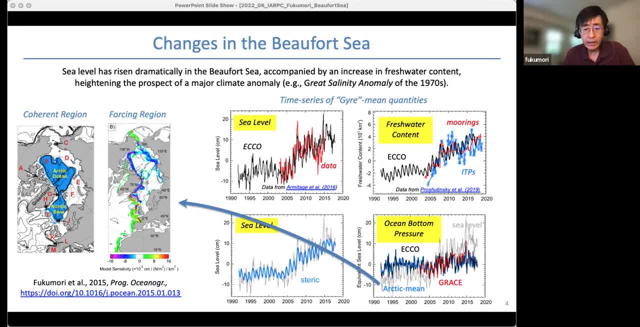 of another IARPC presentation based on the paper at left, and was found to be driven by winds along the continental slope of the Arctic and its neighboring seas away from the Beaufort Sea. Here in this study, we explore the causal mechanisms of these other variations that are unique to Beaufort Sea. 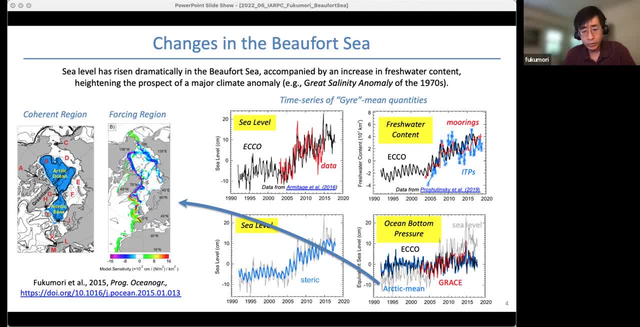 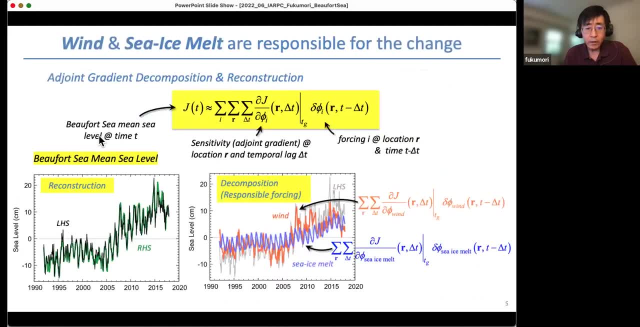 especially its interannual to decadal change. using the ECHO model, Employing what we call the adjoint gradient decomposition, we expand Beaufort Sea's mean sea level j with respect to its forcing phi on the right-hand side. 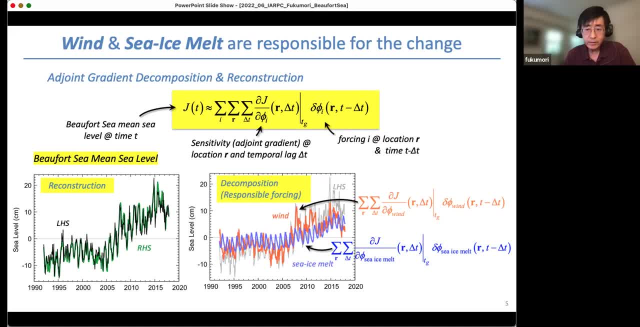 This equation is described as a function of type of forcing, subscript i, like wind and fresh water, flux at the surface, the forcing location r and time lag, delta t between sea level and the forcing. This equation is essentially a first-order Taylor series. 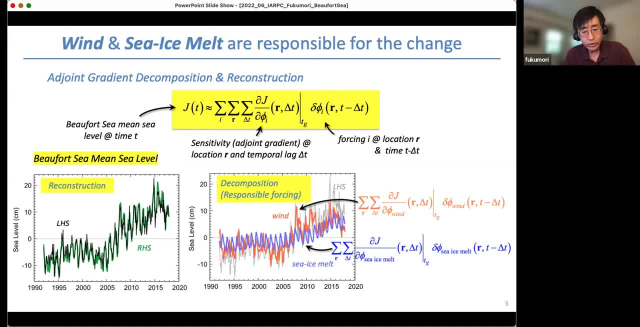 expansion using the model's adjoint to compute the decomposition's gradient coefficients. Importantly, unlike correlation, this equation describes the relationship between the quantity of interest j on the left-hand side and forcing phi on the right-hand side. The left figure at bottom illustrates the skill of this expansion. 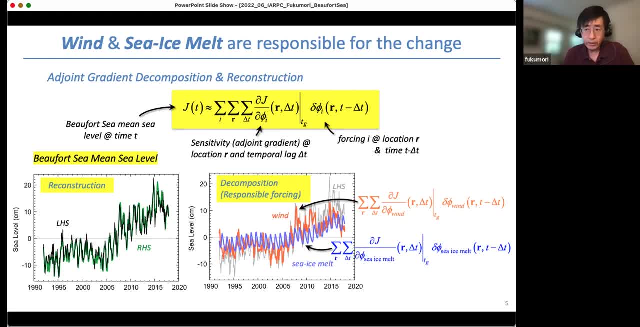 comparing the left-hand side from the model in black with the sum of terms on the right-hand side in green. Now the agreement between the two curves also hinges on the physical consistency of the echo estimate. The right figure compares the dominant components of this expansion. 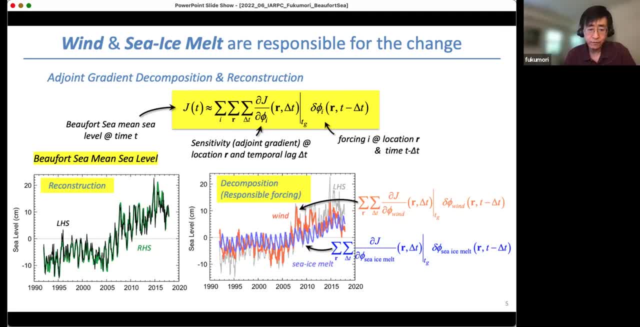 The wind part in orange and the fresh water flux from sea ice melt is shown in blue. Wind accounts for most of the intra-seasonal and inter-annual variation of the model's sea level. that's also shown in gray, Whereas sea ice melt explains the seasonal change. 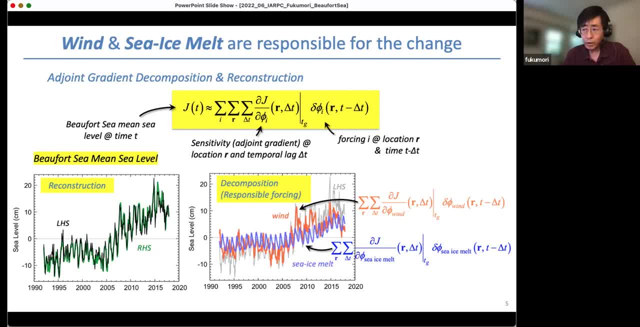 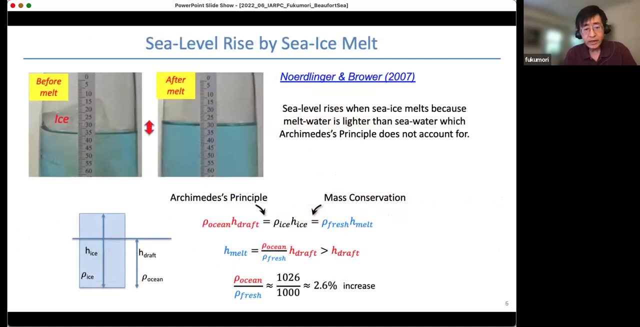 Significantly. however, both are equally important at decadal timescales, as you can see, especially towards the end Now. sea ice melt is often ignored in sea level change, based on Archimedes' principle, But because sea ice is fresher than seawater. 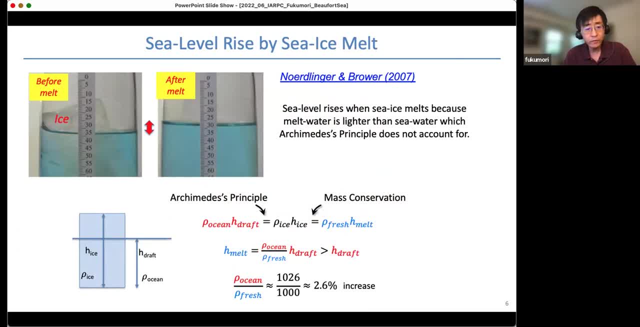 sea ice melt occupies a larger volume than equivalent seawater and causes sea level to rise, as was demonstrated by Nordling's and Brouwer shown here. We'll skip the details, but the melt amounts to a sea level rise of about two and a half percent. 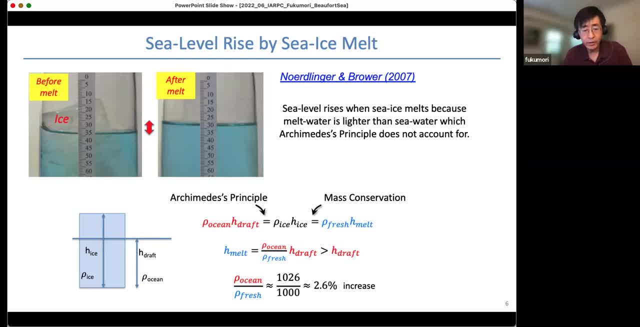 of the melting sea ice's draft. That's the height below the sea surface. This is one reason why sea ice melt matters to Beaufort Sea's sea level. But there are two more factors which are important and we'll get to that shortly. 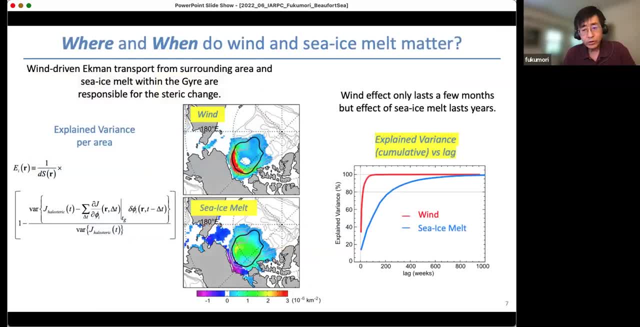 Now the adjuvant decomposition in the previous slide can also tell us where the relative forcings matter and when, which together provide insight into processes at work. For instance, this left panel shows where the forcing matters in terms of the amount of Beaufort Sea's. 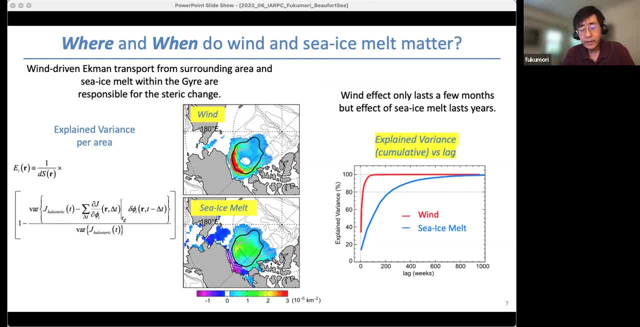 steric sea level variance explained by wind and sea ice melt at different locations. For wind and the top figure, the results indicate its contributions mainly reflect increasing lateral ekman transport of fresh water that's surface-intensified, For instance the dominant contributions from wind. 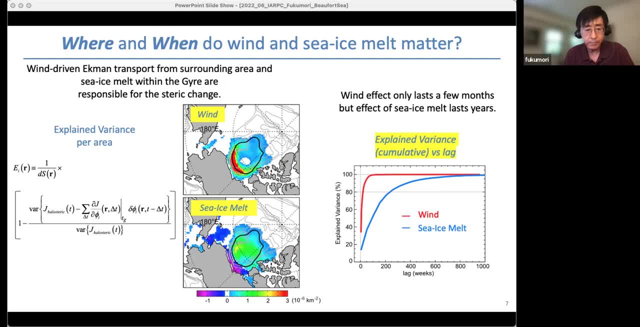 are found primarily along the edge of the domain contoured in black, instead of over the subject region itself, with the largest found along the southern border, over the continental slope, where a change in wind is the largest. Moreover, these contributions come from winds parallel. 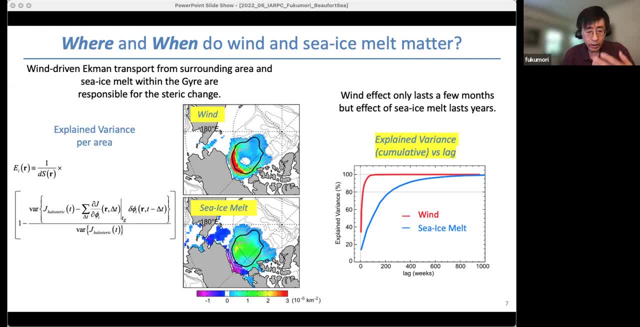 to this region's boundary instead of across it, with clockwise winds around the domain increasing Beaufort Sea's sea level and opposite winds decreasing it, consistent with ekman dynamics. In comparison, the sea ice melt contributes mainly over the Beaufort Sea itself, reflecting the effects of 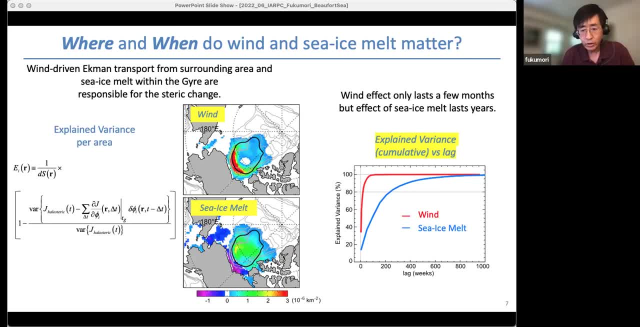 over the region, with additional contributions representing the general pathway of circulation, such as the lateral convergence from neighboring regions associated with the anti-cyclonic Beaufort Gyre and the circulation from the Pacific. The timescale of the two components are also distinct. 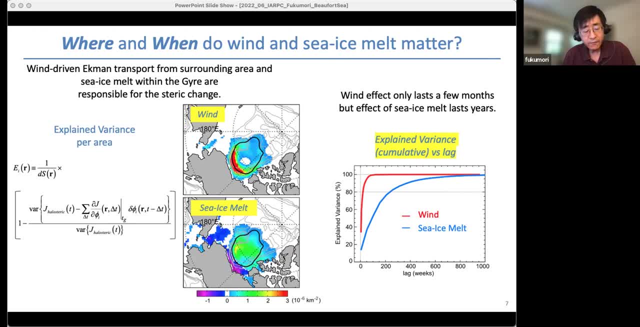 and are shown in the right panel. This is as the variant measured, as the variance of each component. The vertical laufenheit is the time time scale of the gyres and the vertical wave cycle is the time scale of the gyres explained up to different lags. 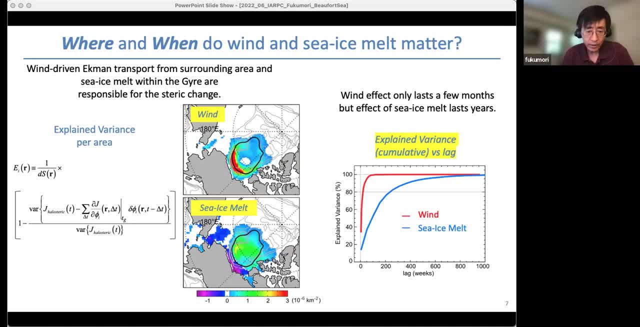 Whereas contributions from wind shown in red only matter up to a few months, effects of sea ice melt in blue have a much longer timescale, lasting years. This time scale difference can be attributed to wind, mainly causing a mechanical deformation of the gyre. 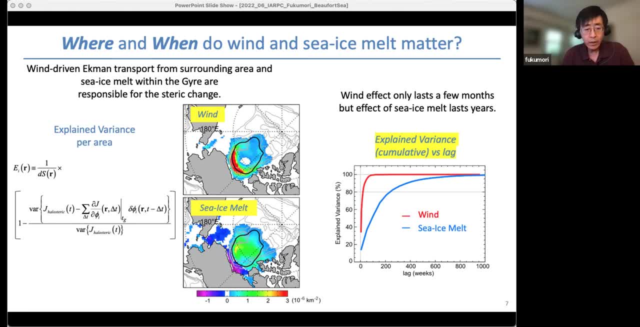 that relaxes in a relatively short amount of time, Whereas any addition of freshwater over the domain lasts much longer because of the semi-closed nature of Beaufort Sea's gyre circulation. So anything that's added to the region keeps circulating within the gyre for years. 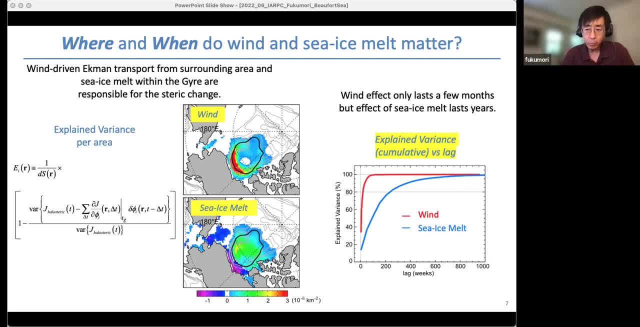 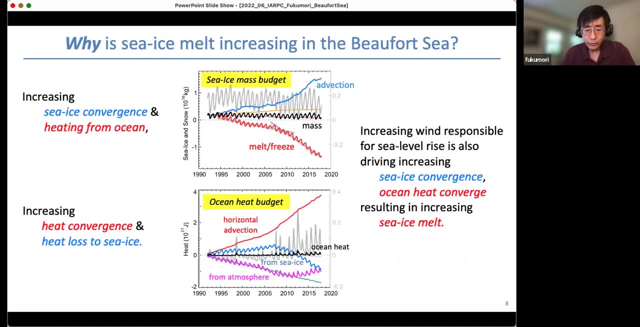 which is the second reason why sea ice melt becomes important for Beaufort Sea's sea level change at long decadal timescales. Finally, we investigate the cause of the increasing sea ice melt by examining the region's budget for sea ice mass and ocean heat content illustrated in this figure. 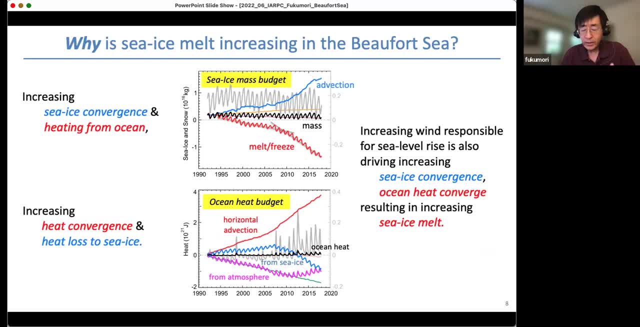 Each figure shows time series of the respective quantity, in black and in different color, the time interval of other terms in the tendency equation which add up to the corresponding black curve. The gray curves are the same as the black ones, but scaled to show details with the axis on the right. 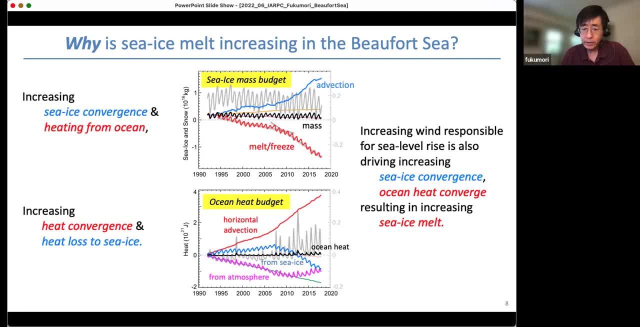 We'd like to draw your attention to the general slope of the curves, the change of slope of the curves, illustrated, for example, by the gray lines fitted to the red sea ice melt in the top figure. This slope change indicates that the sea ice melt. 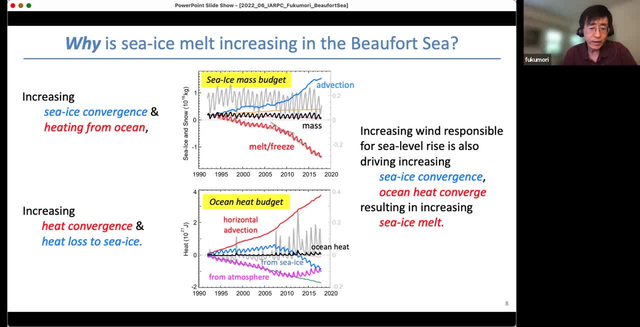 increasing from around 2007,. but this increase isn't balanced by decreasing sea ice in black. Instead, the increasing melt is balanced by the increasing amount of ice that's brought into the region by wind, shown in blue. So the melting sea ice behind increasing sea level. 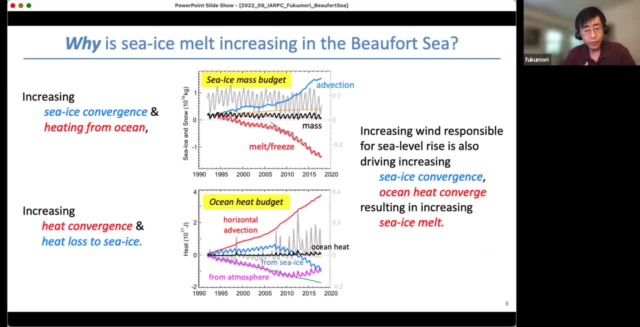 comes from outside the region, not within, which is the third reason why increasing sea ice melt is contributing to Beaufort Sea's sea level rise. This increase in sea ice melt turns out to be due to increased heating from the ocean, as opposed to the atmosphere or direct radiative forcing. 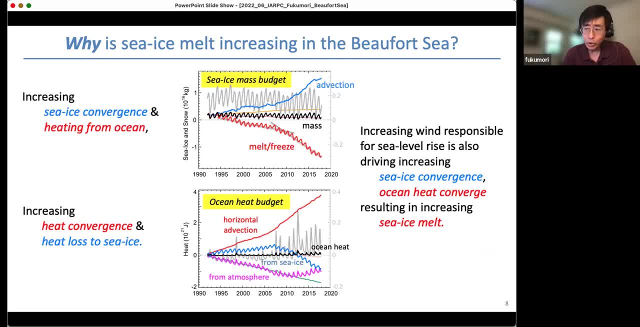 and is reflected in the change of slope of the blue ice ocean heat flux in the ocean's heat budget in the bottom panel. This increased heat that went into melting sea ice melt, however, also didn't come from changing ocean heat content in black. 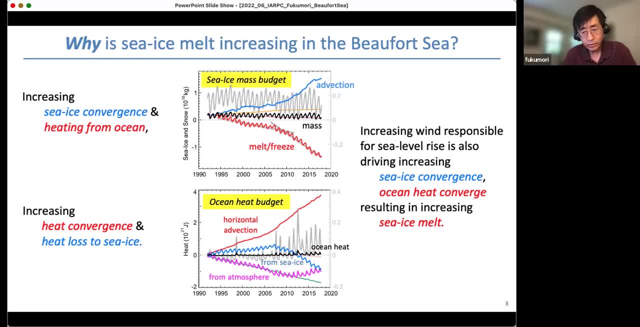 but by the winds increased advection of heat into the region in red and a secondary radiative component in magenta that occurs later. So Beaufort Sea's increasing sea ice melt is primarily due to wind, bringing in more sea ice and more heat, and is a wind driven change. 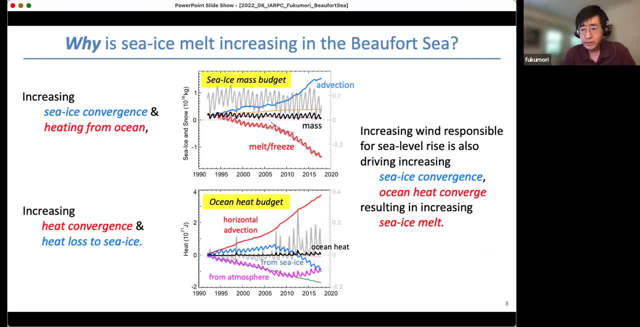 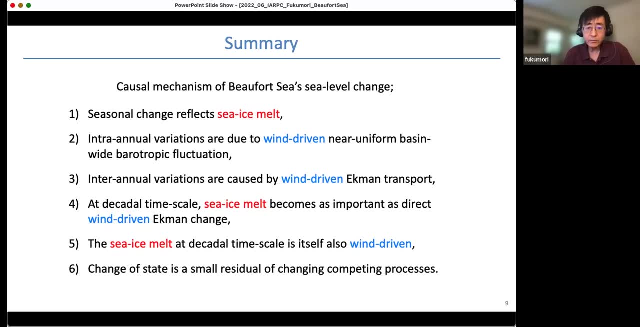 just like the rest of the oceans, respectively, And this is the result of the ocean's response underlying its sea level rise. So, in summary, our study suggests Beaufort Sea's sea level is driven by wind and sea ice melt. Sea ice melt dictates seasonal change. 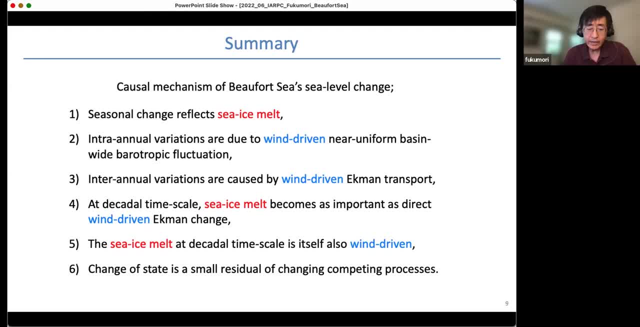 and wind dominates other intra-annual and inter-annual variations, but both contribute equally at decadal time scales. Importantly, the decadal change of sea ice melt is itself primarily wind driven. Finally, this analysis shows how change in Beaufort Sea state 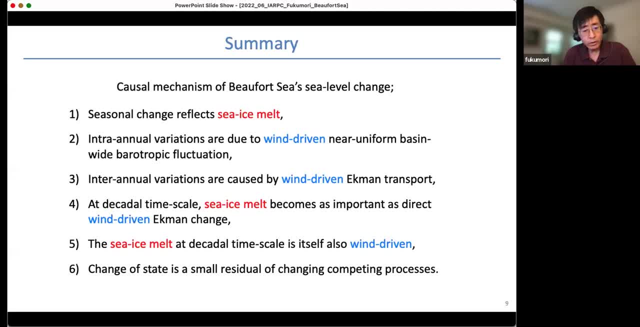 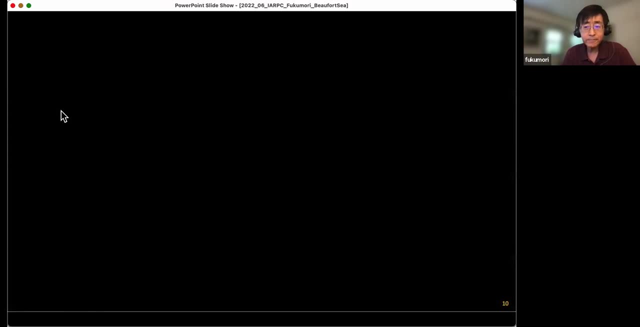 like the ocean often is, is only a small residual of much larger changes in competing processes and illustrates the importance of resolving those processes to understanding what's happening. And with that I'll end my talk, Thank you. Thank you Very nice, Ishiro. 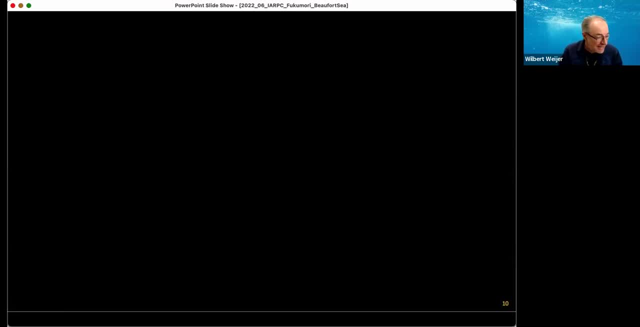 Thank you very much. This was a very fascinating presentation. I think we have maybe eight or seven minutes. seven or eight minutes for some clarifying questions from the audience. Anybody has a question for Ishiro? you can also put it in a chat. 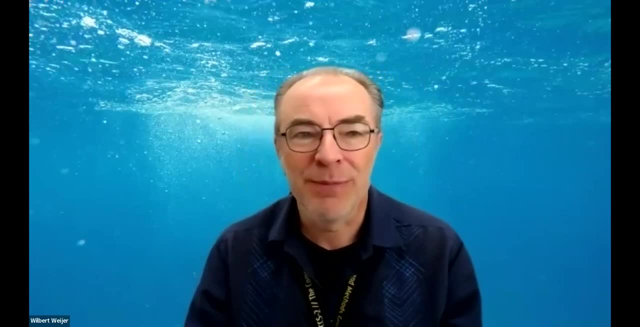 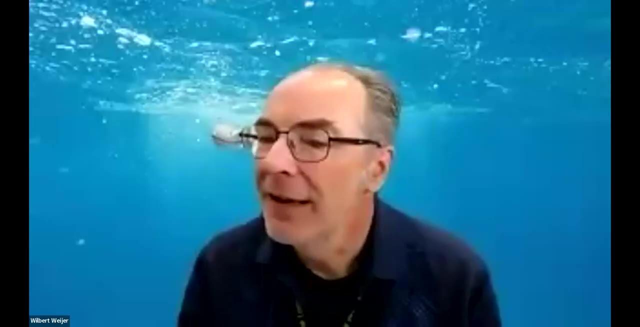 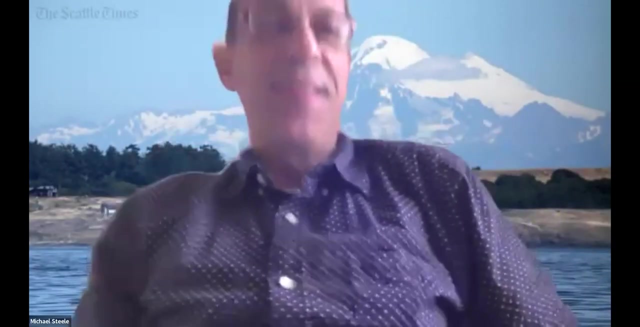 but if somebody wants to speak up to ask a question, that would be great. Well, Brett, there are two hands raised, Three hands raised. I think Michael Steele is the first. but, yep, Thanks, Okay, Yeah, my connection is lasting. 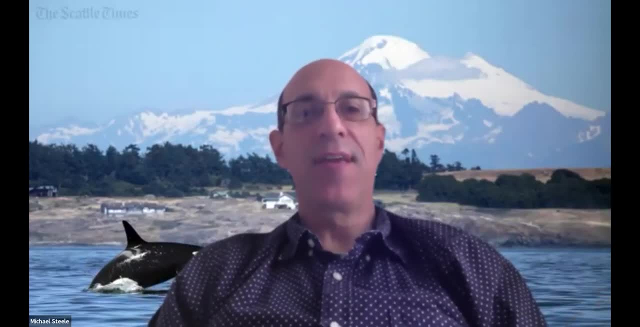 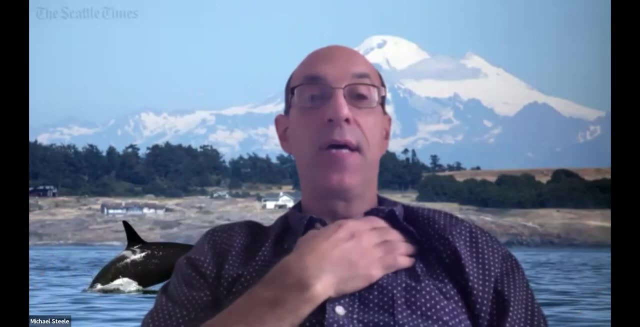 So that was a super interesting talk, Thank you. So my question is: I'm a little confused by the stuff at the end. Probably you had to rush it, but the ice is melting because of the atmosphere. Can you explain that a little more? 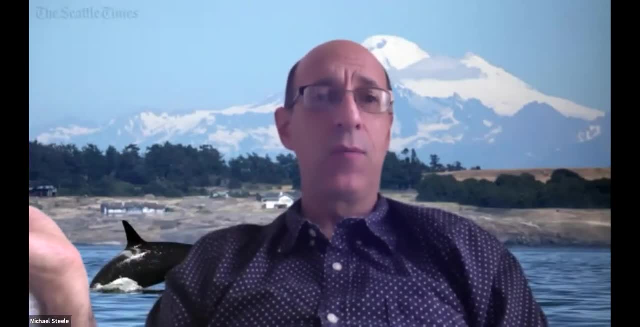 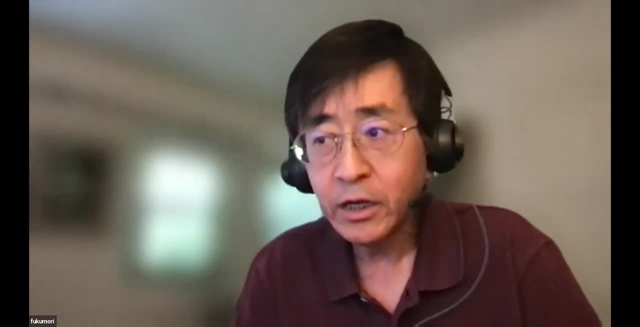 Is it? there's warm air advection coming in. I mean, what is that about? Ice is melting because of the ocean. It's because it's getting heat from the ocean. So what I didn't show is the sea ice heat budget. 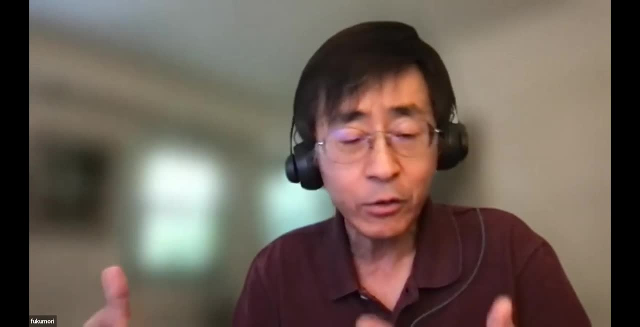 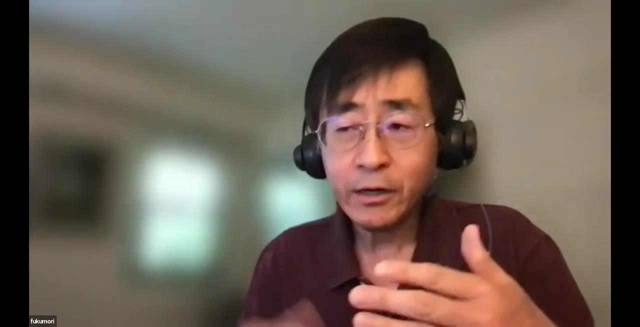 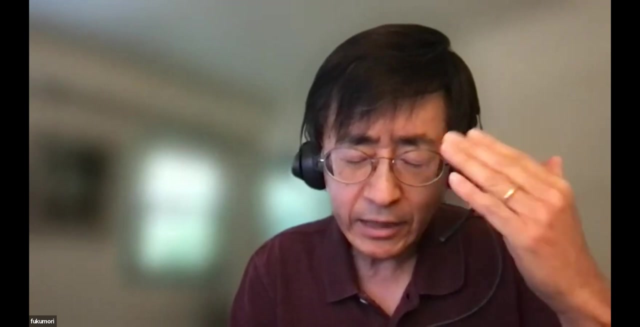 And so ice is of course melting by gaining or losing heat to the atmosphere or the ocean. And the plot that I haven't shown, which I do have a plot somewhere in this slide of decks, deck of slides: the ice, atmosphere, heat flux. 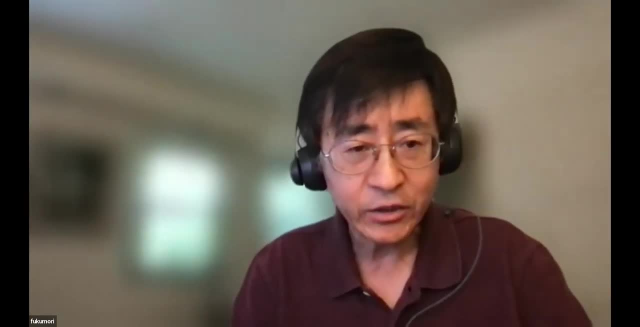 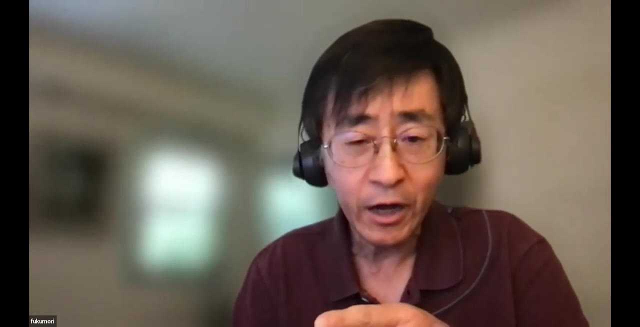 the same plot is basically a straight line, Whereas the ice ocean heat flux. there's a bend in the curve, There's a break in the slope And that is the same shape as this blue curve on the bottom. So the heat that melts the ice. 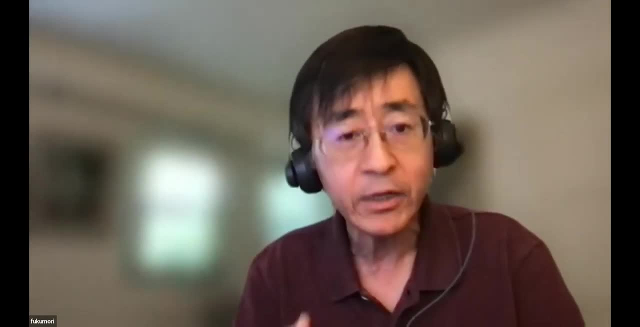 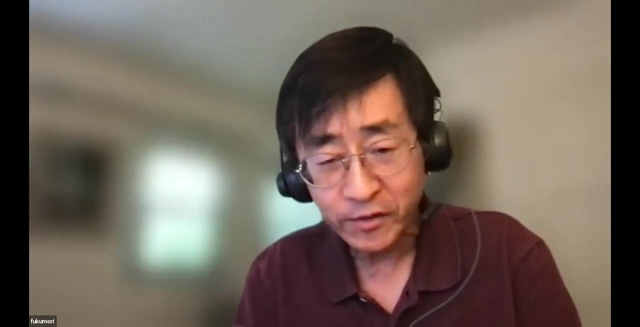 it increased heat that's accelerating the sea. ice melt is coming from the ocean. Now that heat that comes from the ocean is not really changing the heat content of the ocean that much. as you see here, the black curve curve is pretty much flat. That extra heat is actually brought in by the wind. That's 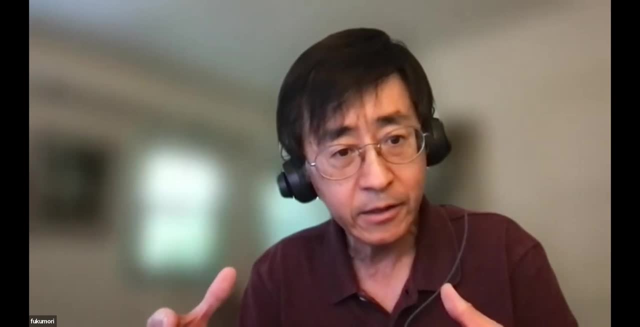 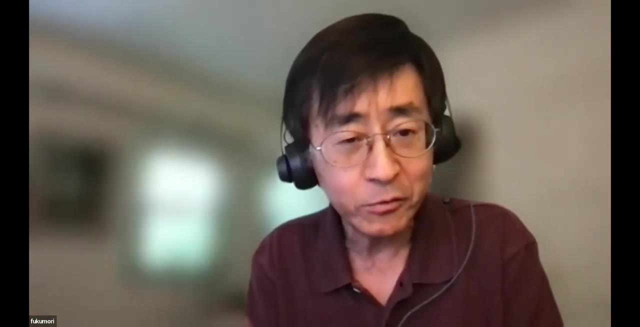 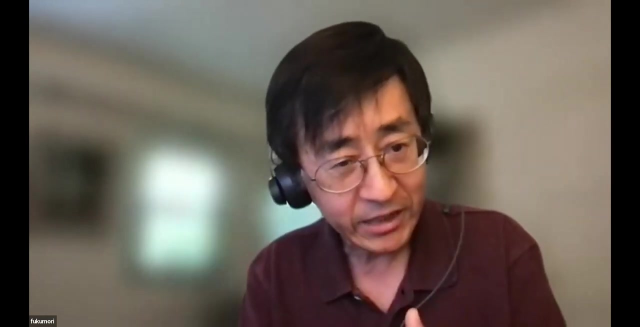 the red curve, the horizontal convergence of heat from the surrounding. So the wind is bringing in extra ice and extra heat and it's all melting within the Beaufort gyre And because the gyre is closed, it's going to stay there and it accumulates, Even though. 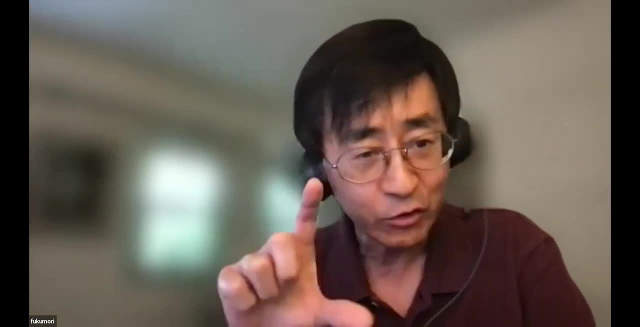 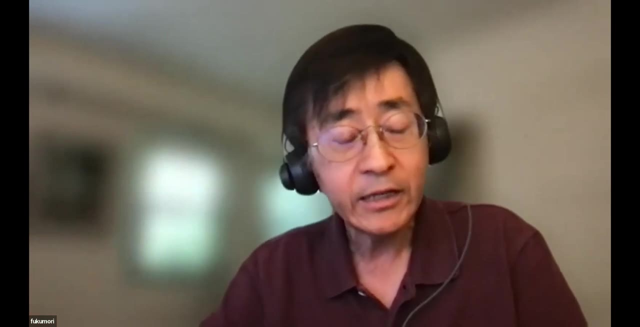 the sea level rise by sea ice melt is only two and a half percent of the draft. it keeps on accumulating And over time, over decadal timescales. you begin to see it. That's what we think is happening, At least that's what seems to be happening in the echo analysis. 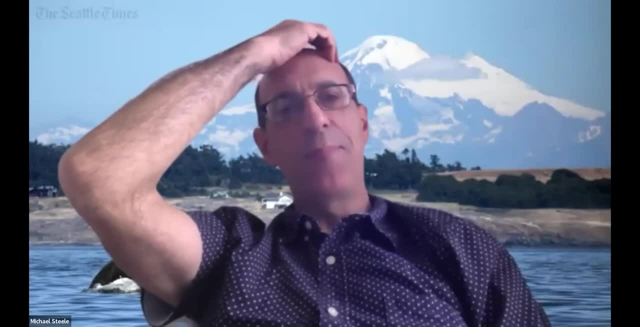 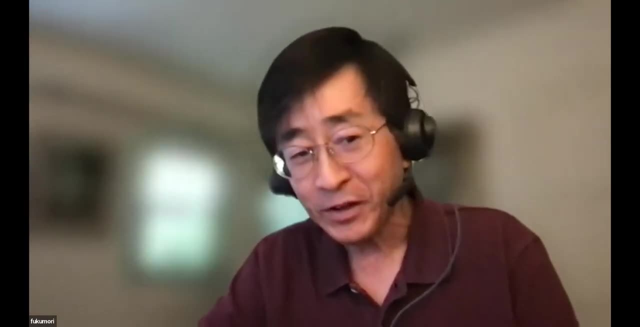 I see a lot of hands. I see a lot of other raised hands, so I'm going to bow, but I'm honestly, I'm sorry, I'm a little still confused. OK, so I'll be happy to come back to that. OK, you've got time. 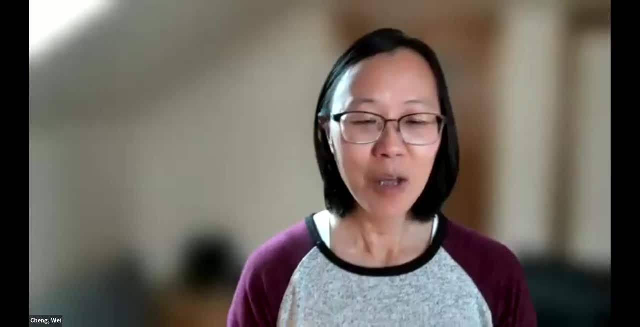 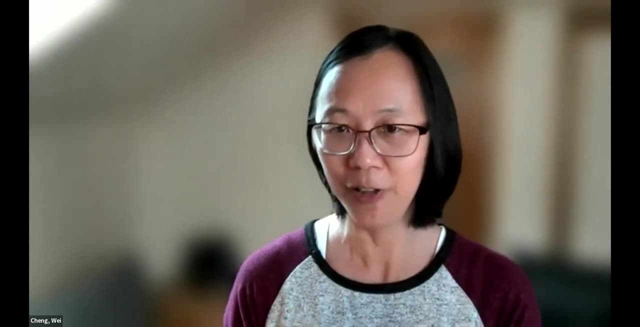 And Wei. Sorry, my question relates to the. at the start of your talk In your slide you showed a panarctic versus Beaufort gyre kind of the difference- And then you said something about the panarctic is due to the wind around the boundary of. 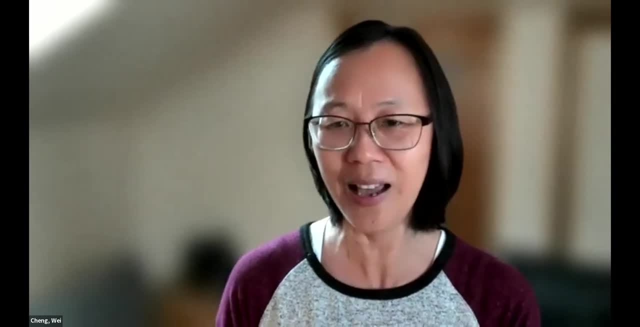 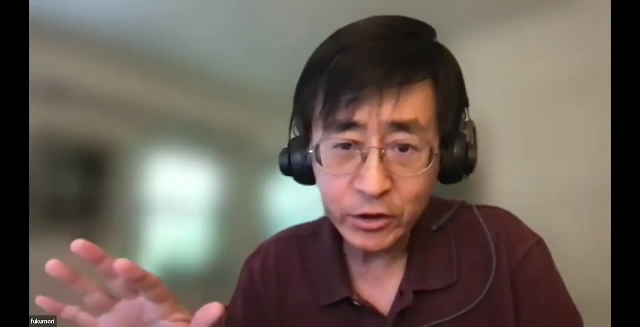 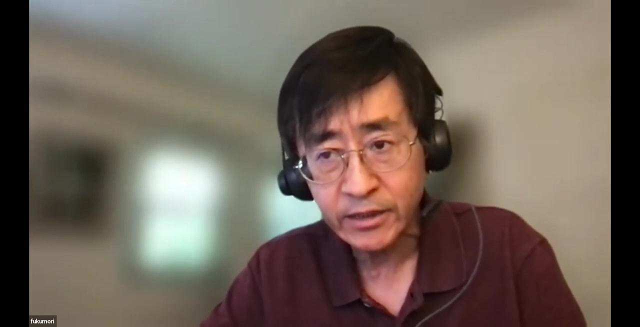 the Arctic. And then- so that that statement kind of confused me a bit- I wonder: Yeah, Yeah, this, they? there's two things, many things going on. One thing I tried to separate is the, this barotropic, the deep ocean signal, the high frequency signal, which causes this. 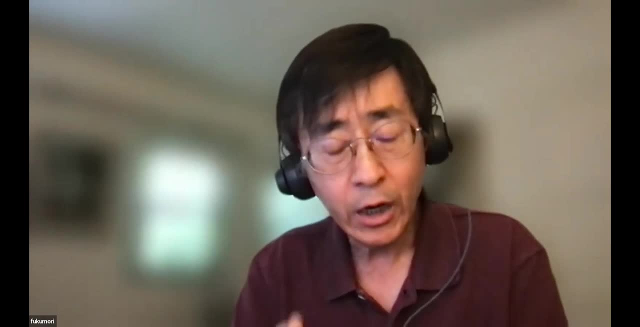 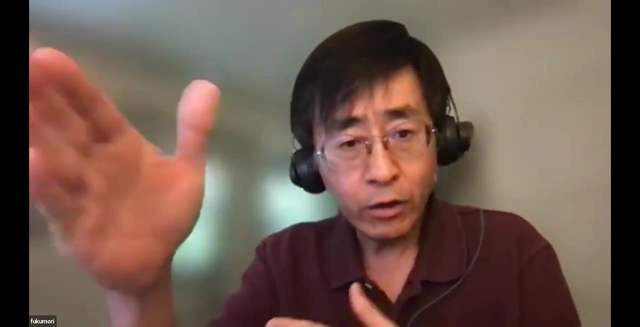 this ocean bottom pressure or sea level, a uniform up and down which was initially found by data by Cecilia Peralta-Ferriz and her colleagues across the Arctic deep ocean, basins of the Arctic Ocean and the Nordic seas illustrated in the left panel, This blue. 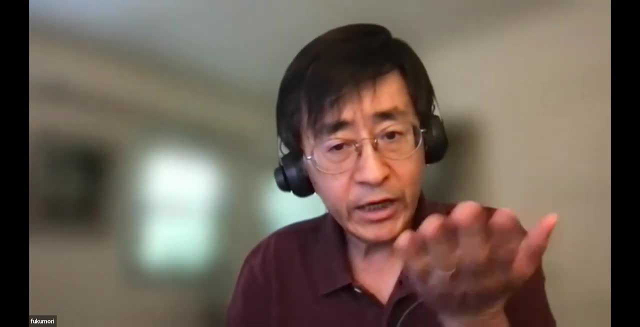 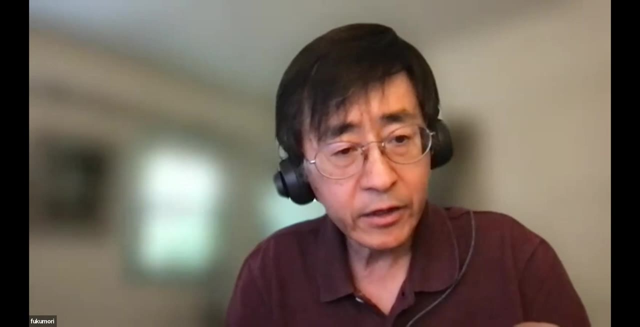 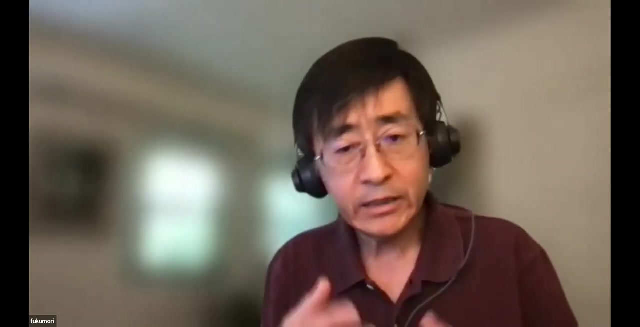 region, although I just colored it. if you look at sea level, it goes up and down uniformly And that is caused by winds, shown in the right panel- on the continental slope of the Arctic And the North Atlantic and a little bit of elsewhere. And this is what's happening is. 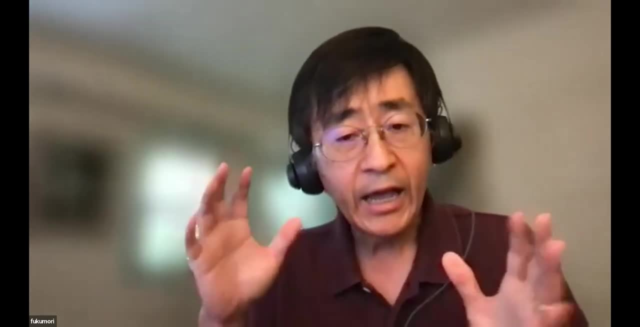 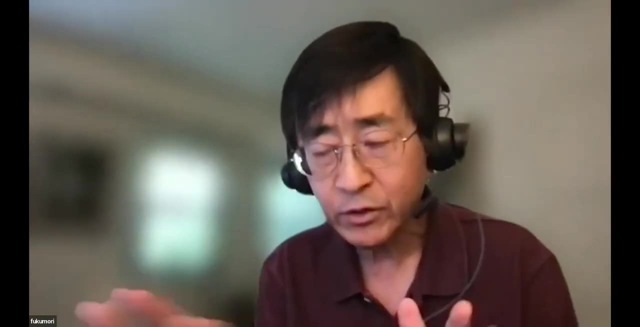 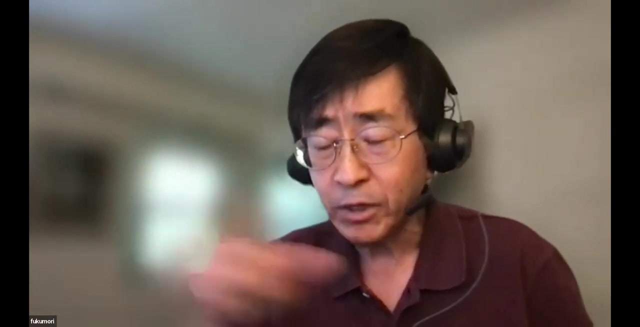 closely trapped waves generated by these these winds, And it's an entirely different phenomena from the decadal change that we see in the Arctic Ocean, And so the high frequency part is due to this continental slope: winds all around, And what's left is this, essentially: 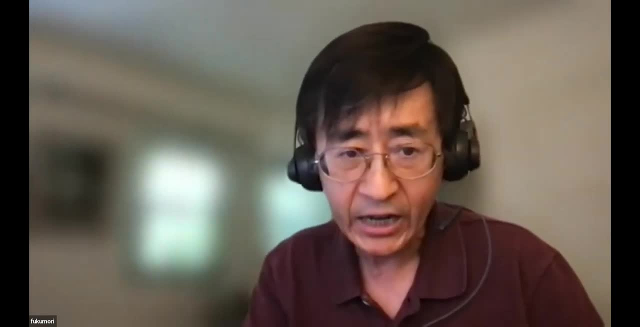 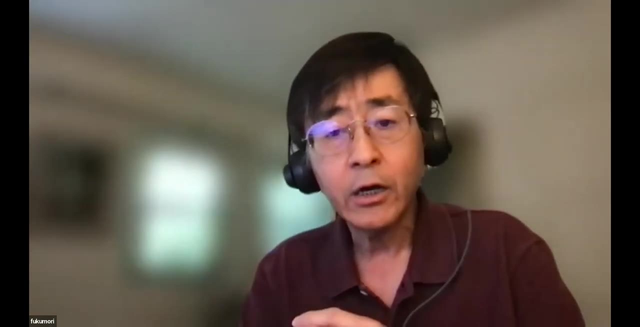 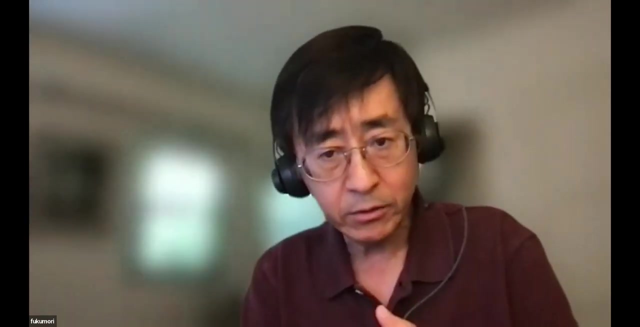 the blue steric sea level change, this annual and inter-annual and decadal change- And that's the main subject of this talk, which was due to local winds, Ekman-Trans convergence and divergence and sea ice melt. Does that make sense? 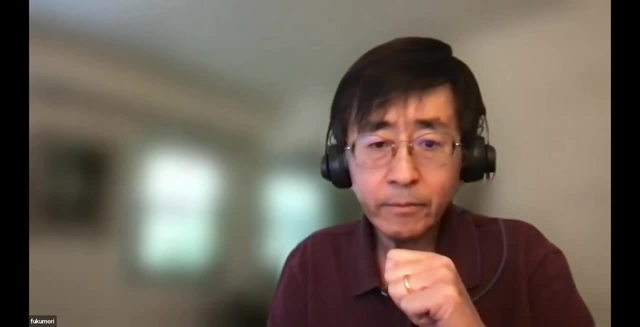 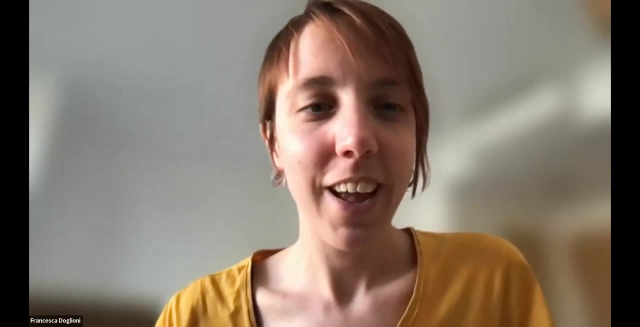 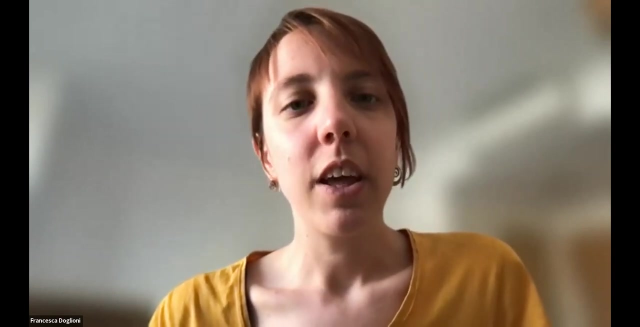 Francesca, Yeah, if you still have time. I mean, I think my question is along the line. So I was wondering how can you distinguish the effect of wind and sea ice? Because if you remove wind, as you say, you 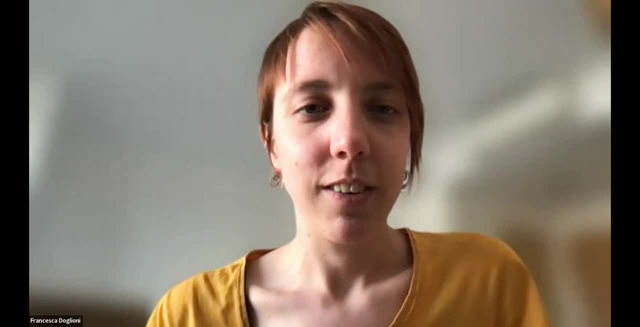 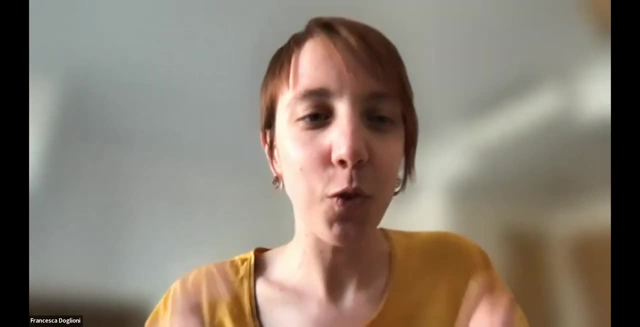 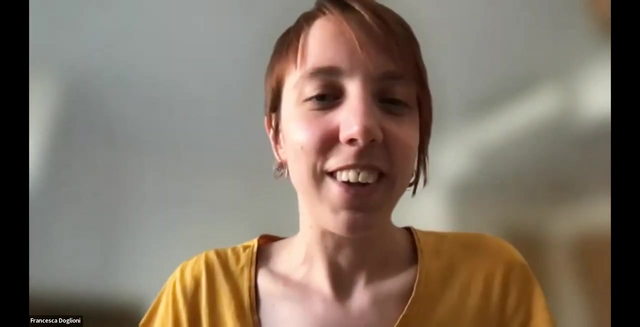 wouldn't have convergence, So you couldn't say that it's the sea ice melt that is contributing. So yeah, there was my question And also I think I was a bit confused by the picture of the sea ice in the glass because I tried to do that experiment myself. So yeah, but 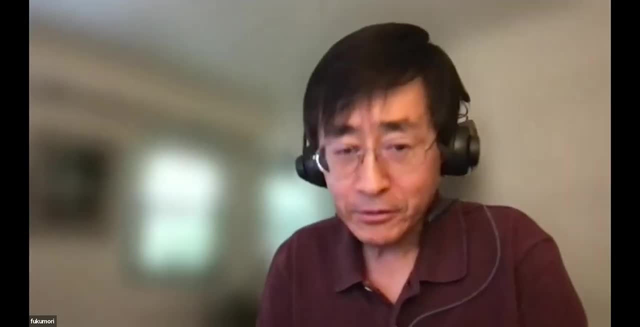 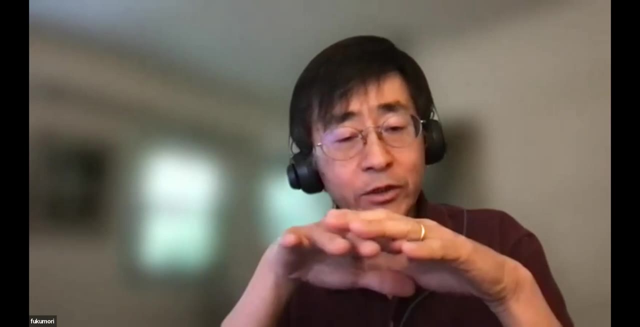 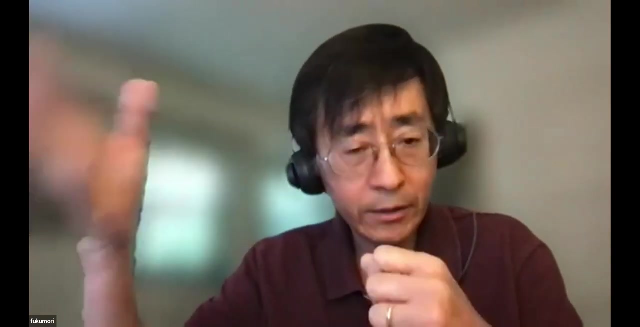 that's probably the Okay. yeah, I'll address both questions. We can separate this because what we do essentially is we just take the ocean model of this coupled model And when we ran ECHO, the full coupled model, we save the ocean surface forcing wind. 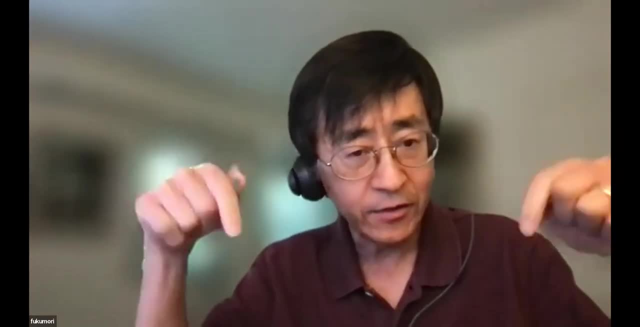 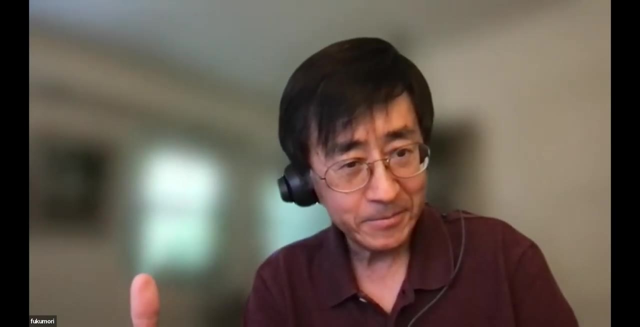 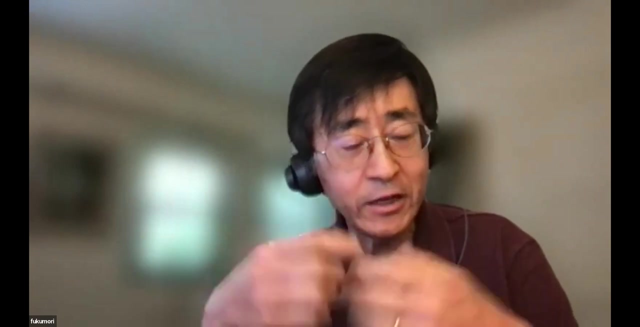 stress, heat flux and fresh water flux acting on the liquid surface of the ocean, And we just run the ocean model with that. Okay, So we can then essentially tell which part is due to wind, which part due to fresh water flux. fresh water flux does change, as you pointed out, when sea ice moves, but that's. 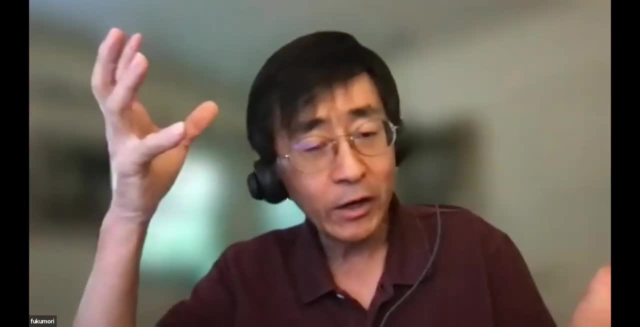 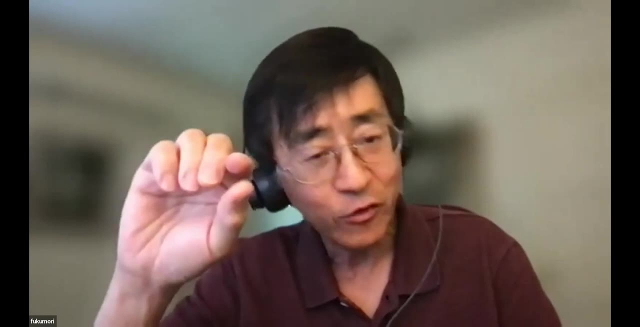 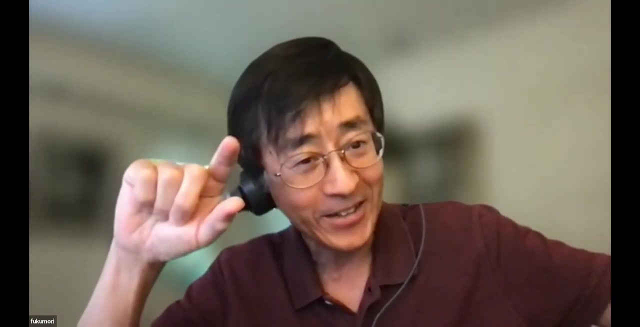 taken out already. we've separated that because the that sea ice impact on the ice is basically through heat and fresh water exchange And that's the fresh water and heat flux that we are forcing the ocean. So even if we switch off wind, there's still that effect of the. 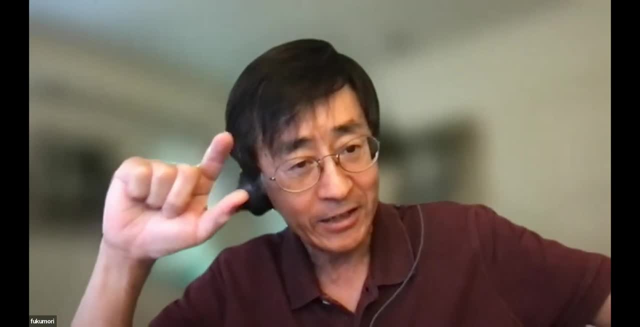 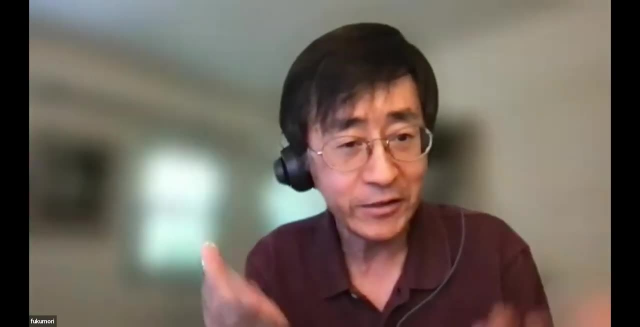 cold, the cold, the cold of fresh water and and heat flux. that would have happened if the ice were there. but the ocean doesn't know that. the ice is not there. You only cares what the flux is. So that's why we separate how we separate the two effects. 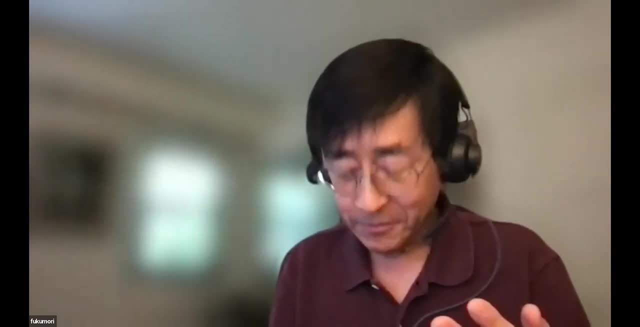 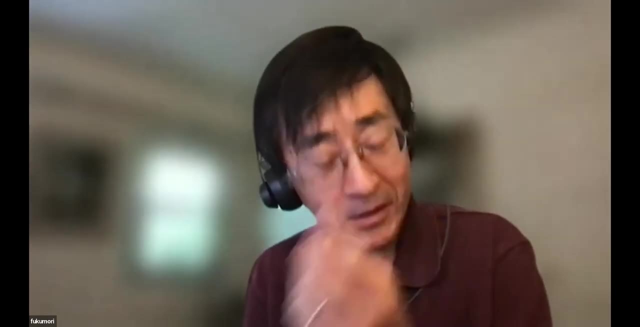 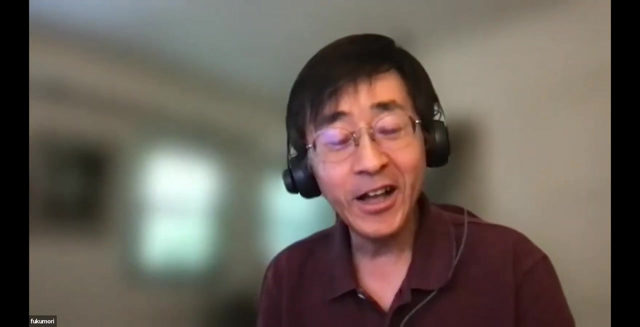 Now going. The other question is the: is the this, this experiment? this experiment, I think, is this picture, I think is brilliant, But they comment on this in this paper. This is extremely salty water to see this effect at this scale. I forgot what the numbers are. 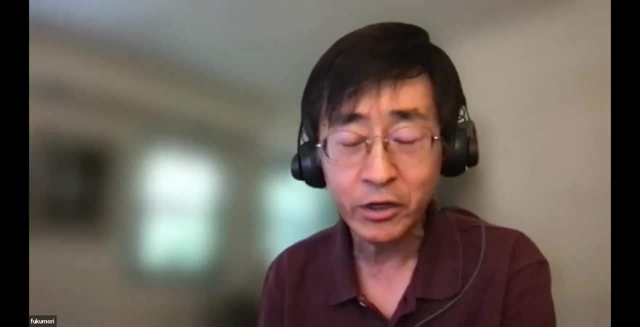 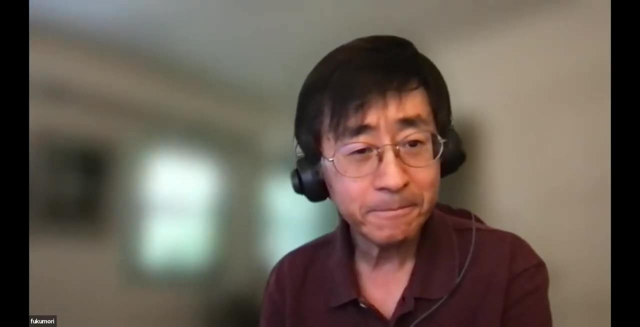 but this is not really seawater. This is a much saltier water And if you do this, yes, you can see the effect like that sea level will go up. So try putting in more salt in the water part when you next time you do this. 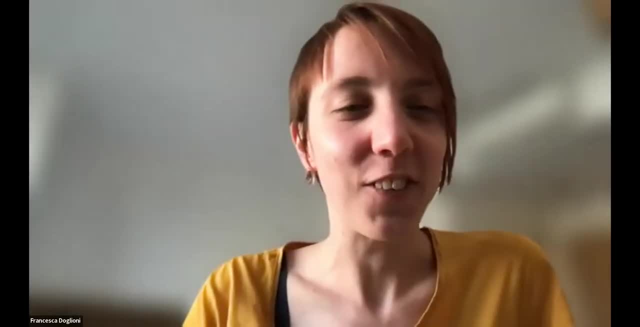 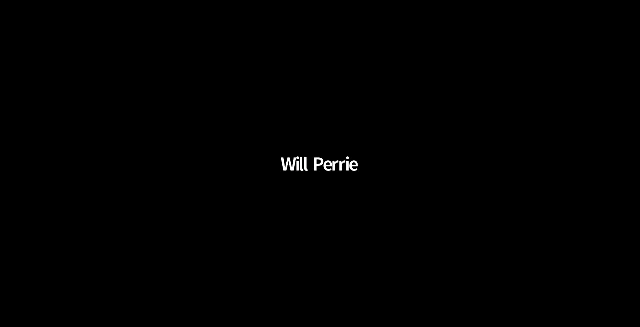 I will try. I still have to figure it out, but I will try. Great thank you. Great discussion. I don't see any more hands raised. I thought John had his hands raised. Do you still wanna ask a question, John, or are you good? 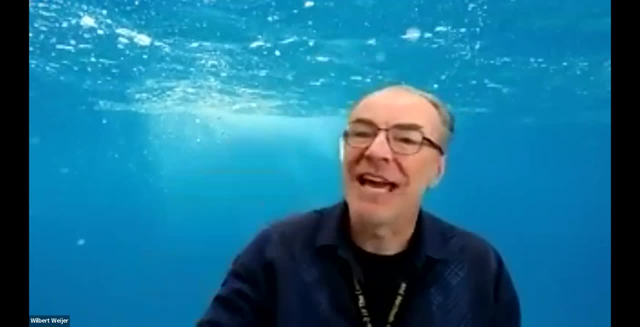 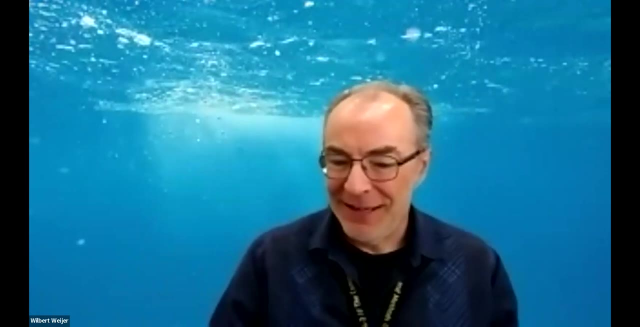 All right, if not, then yeah, you can continue asking questions in the chat also, But for now let's move over to Francesca Dolioni from the Alfred Regner Institute, So I'm pleased to have her here. Thanks, It's quite late. 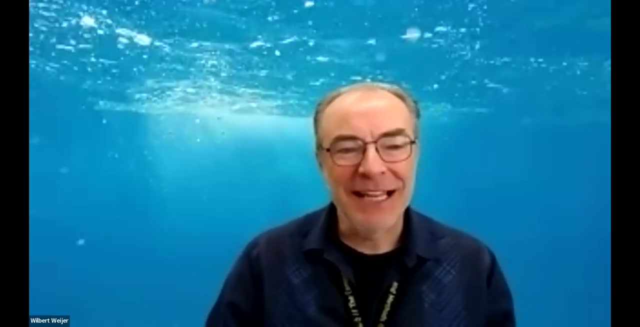 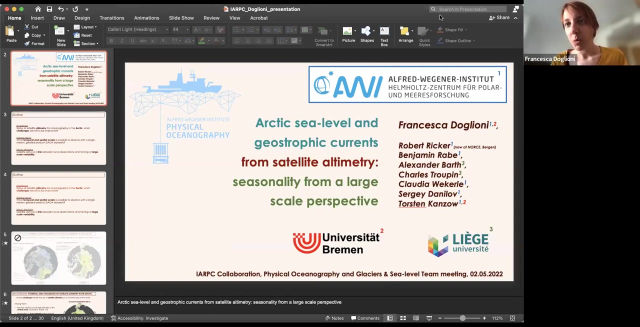 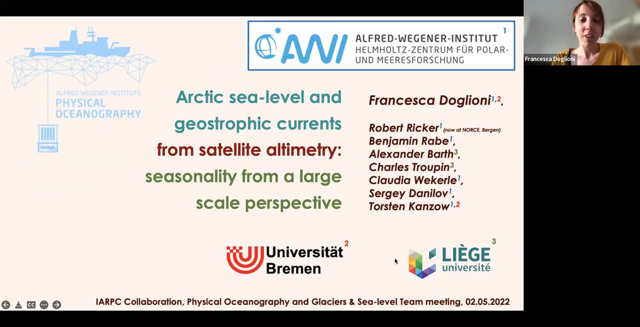 Is it too late there? Probably Still okay. Okay, still awake, that's good. Yep: Sea level and geostrophic currents derived from satellite altimetry. Yeah, so there we go. Maybe just So. first of all, thanks for the invitation. 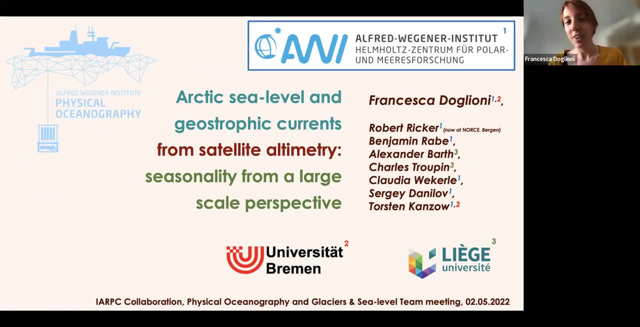 I'm really happy to contribute to this discussion And what I wanted to present today is bits and pieces from my PhD work which I thought fit very well with this discussion. And yeah, on the right side you can see a few of the colleagues. 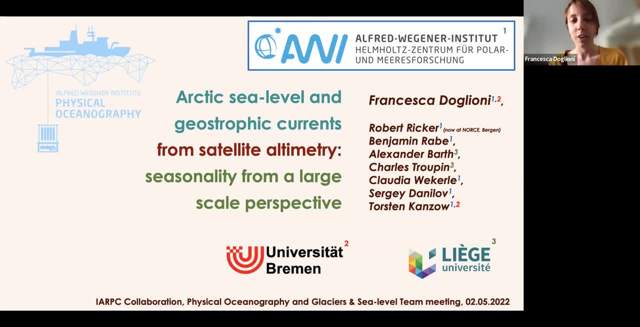 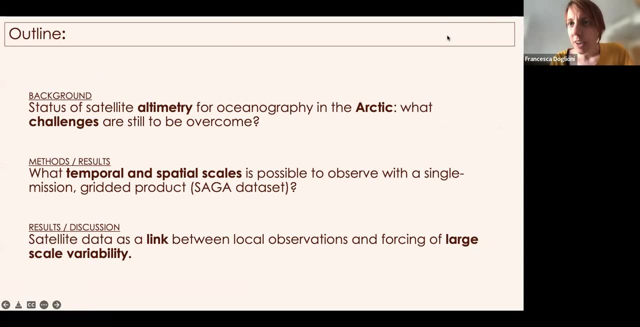 that contributed to my research And yeah, and so what I will focus today? I wanted to focus on three points or three questions. So first let's see. first I wanted to give an overview of what's the status of altimetry in the Arctic. 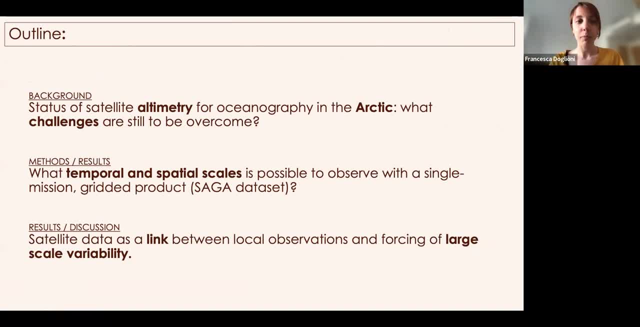 And what are the challenges that still need to be overcome, especially from my point of view? let's say, And that. so I will present a data set, a graded data set that I have generated during my PhD time and show some results to explain. 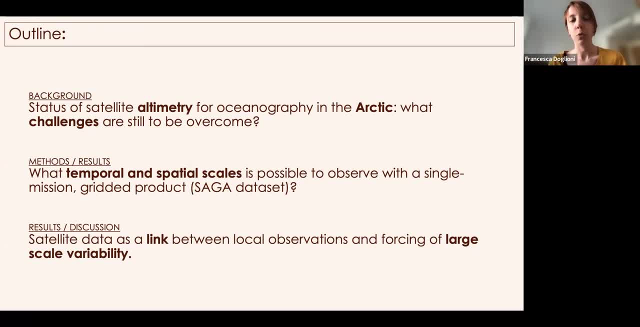 What kind of temporal and spatial scales we can expect from such a data set. And finally, I wanted to have a bit of a discussion of whether this kind of data- satellite data, altimetry data- can be used to link local observations and C2. 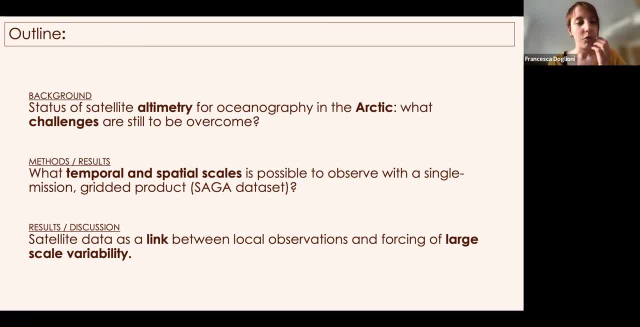 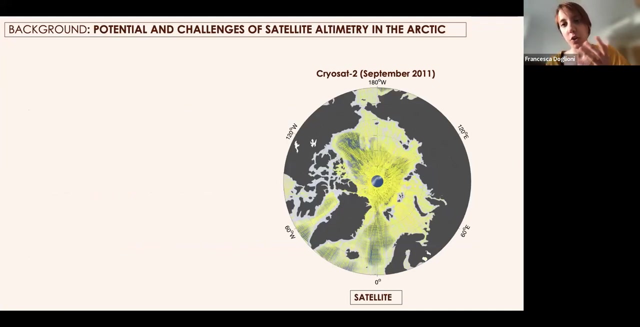 observations to rather large scale variability in surface currents and sea level, Yeah, and also to facilitate understanding the forcing of this variability. And so we can start with the first question. And to start, I would like to show you this figure which shows the actual coverage. 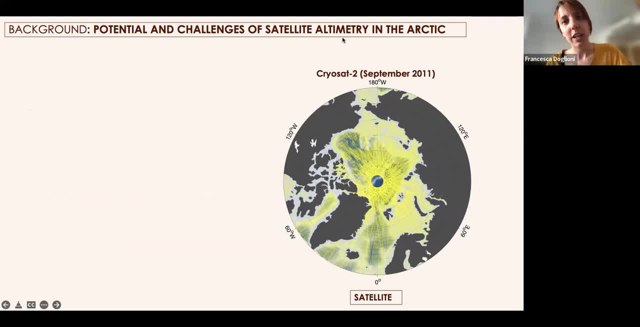 of the satellite altimetry mission CryoSat-2 over a single month in September 2011.. And what this clearly shows is that there is a potential for this kind of data to really fill this somehow, this data gap that there is in the Arctic. 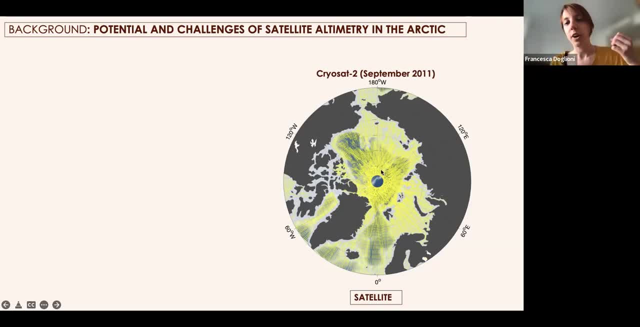 You can see, there is a lot of observation on the shelves in the central Arctic and also under the ice, where actually the satellite can see the sea level in between, in cracks in the ice, And that's how this is derived. But in my opinion there are still several challenges. 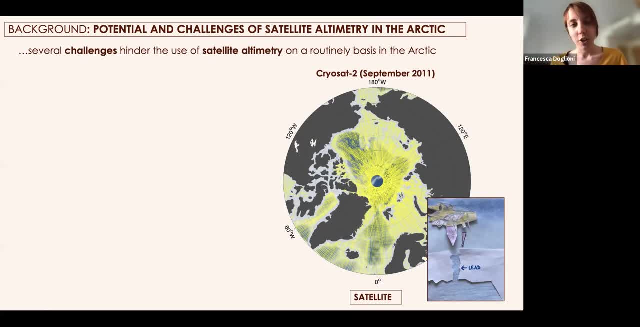 to satellite altimetry, And I mentioned here a few, Which I think is there are a few missions that cover this high latitude And they are discontinuous. Some, for instance IceSat-1, stopped before CryoSat-2. 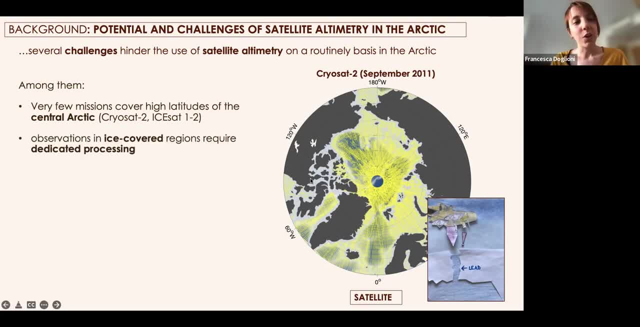 or was very short in time, And then the observation in the ice covered part require dedicated processing. So actually often, especially for oceanographic purposes, they are not really used. And then this is a very important point, that in the Arctic there is very high frequency. 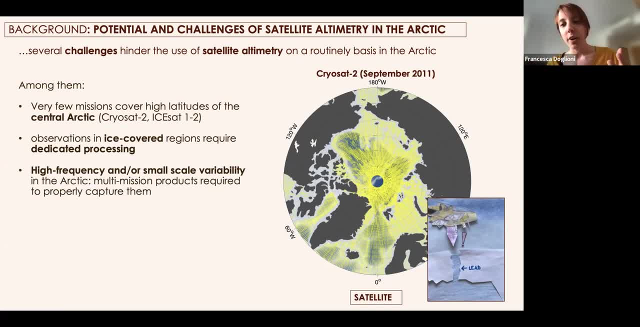 response scale variability, which actually require higher temporal resolution, so multi-mission products to really capture this variability. And finally, these are long-track data And And And for long-term climate studies, as you have seen from Ichiro's presentation as well. 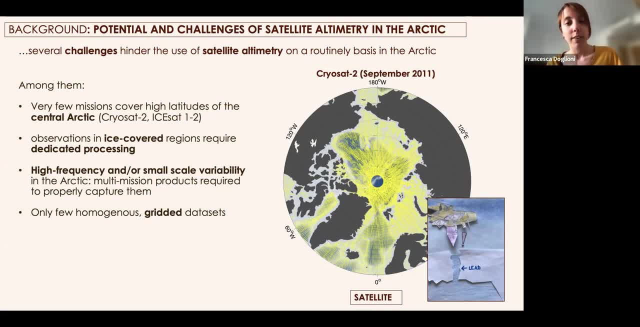 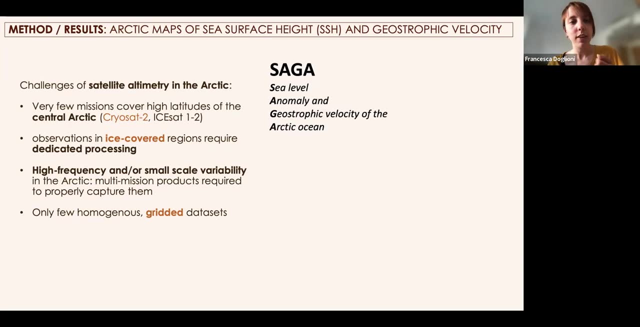 one needs the gridded data sets, And these are still very few, And, for instance, the data set from Armitage has been used so many times, And so in my work I just tackled a few of these points And I generated myself a data set of sea level anomaly. 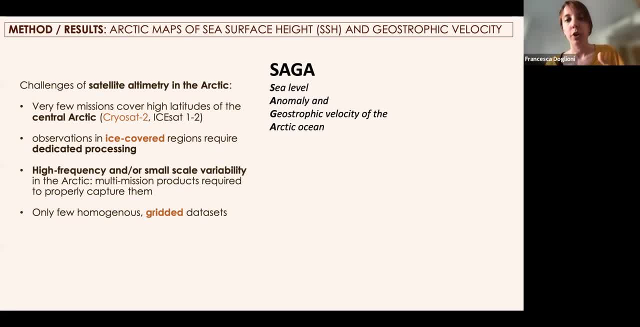 or sea surface height and geosophic velocity for the Arctic Ocean, And I've used data from a CRISR2 mission, so up to 88 north, as you have seen in the previous figure, And then I included also ice cover regions. 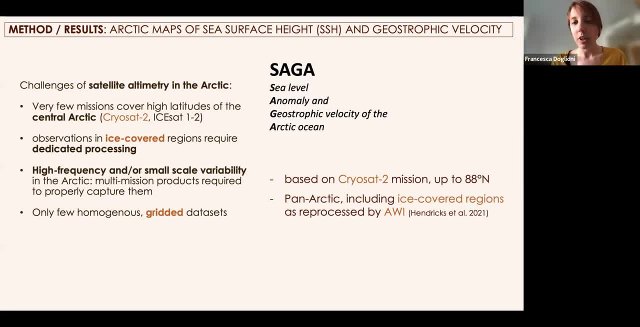 Data from ice cover regions were processed by the Alfred Beckner Institute And I mapped them into monthly maps between 2011 and 2020.. And this data set is now under review, together with the associated manuscript, And And hopefully will be available soon. 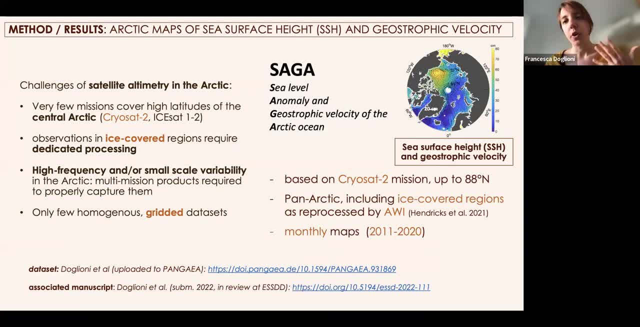 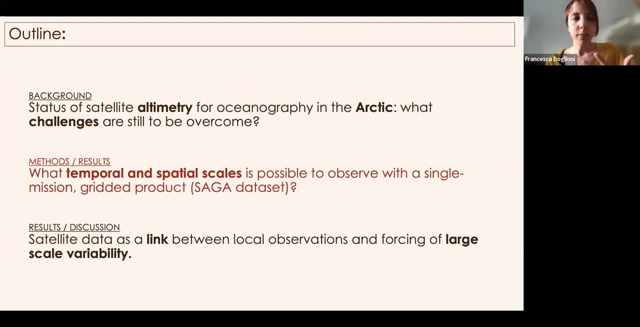 And this is just an example of one monthly map where you can see the actual sea surface side, let's call it the dynamic ocean topography, and the associated geosophic flow. And so this was what I think are still the challenges. 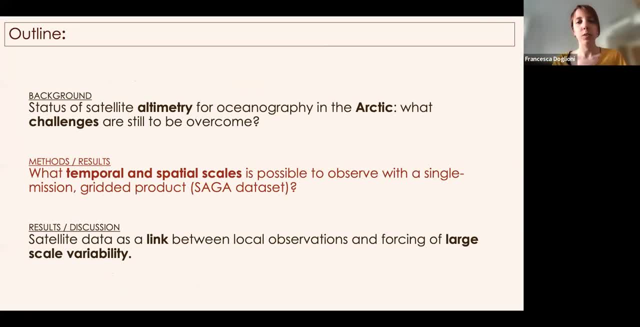 as I said, but then still from a data set that is based on a single mission, as the one that I just presented, this Saga data set, as I call it. What kind of resolution can we expect? What can we observe from this kind of data? 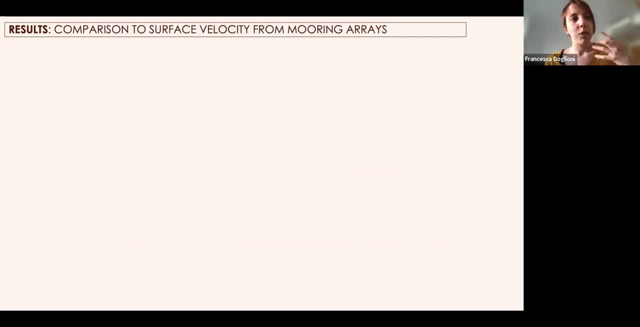 And among the several comparisons that I did to validate this data set, I want to focus here on one validation, which is a comparison of geosophic velocities to mooring arrays, so to velocity, in-situ velocity, for two mooring arrays in the Arctic. 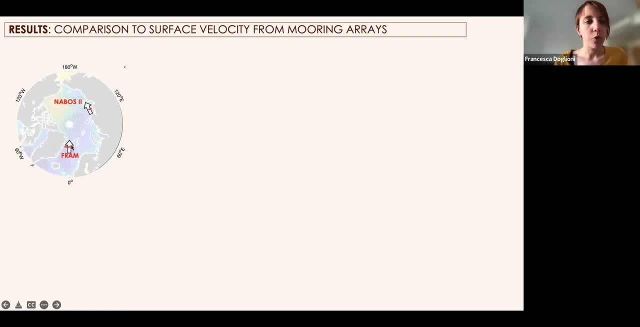 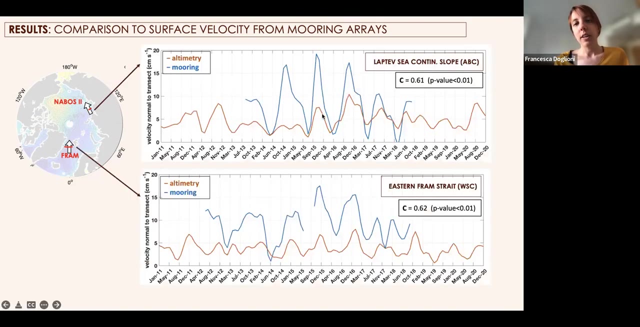 One is in the Fromm Strait And in particular I will show time series of the West Pittsburgh current, And one is in the Laptop Sea continental slope, where I compared velocities in the Arctic boundary current And what we can see is that the two data set agree relatively. 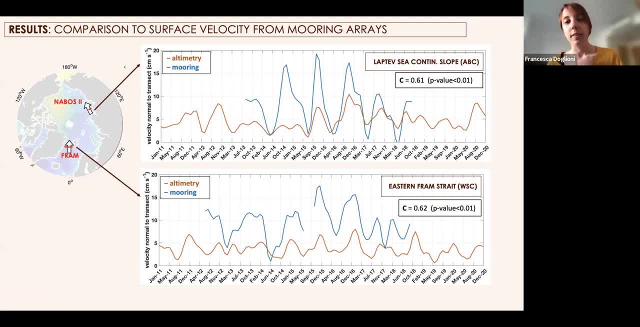 well, And especially, they do resolve both seasonality, seasonal acceleration in the winter period and deceleration in summer. And then, starting from these very local results, can we have a look more at the large scale? What can we see? 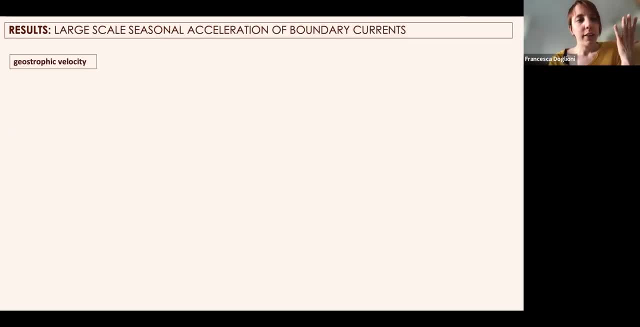 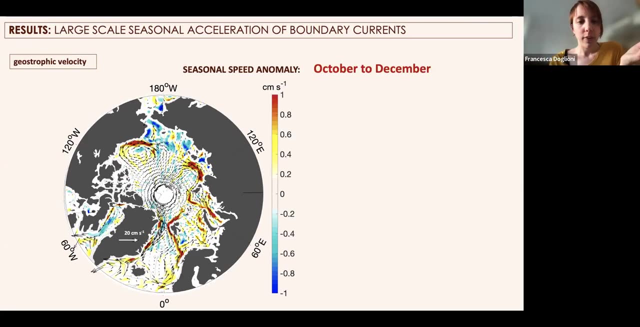 And so if we look at the geosophic velocity in the Arctic-wide, And so if we look at the geosophic velocity in the Arctic-wide, we can see that the geosophic velocity in the Arctic-wide is more than the geosophic velocity in the Arctic-wide. 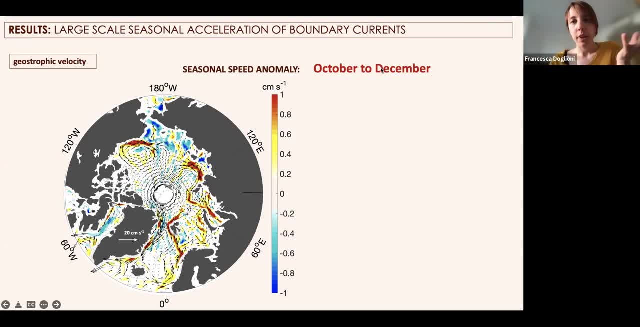 So this is a very interesting domain And here, in the specific, I want to focus on a seasonal speed anomaly. in the period between October and December We observed that there is a large scale acceleration of slope currents, especially in the Eurasian part. 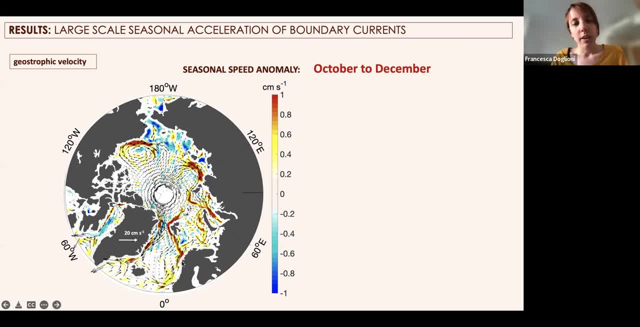 Then there are other processes, for instance in the Beaufort region, where there is a large scale pattern on the Eurasian side, that it's very evident And in a way this result is consistent with many Mooring-inferred results. 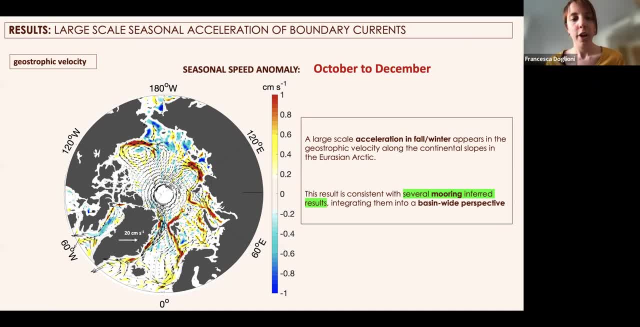 from several papers from previous literature, And here I just put locations where these other studies, for example, show an acceleration of currents or volume transport in early wintertime, let's say, And so from this result we can take that this kind of data can be used. 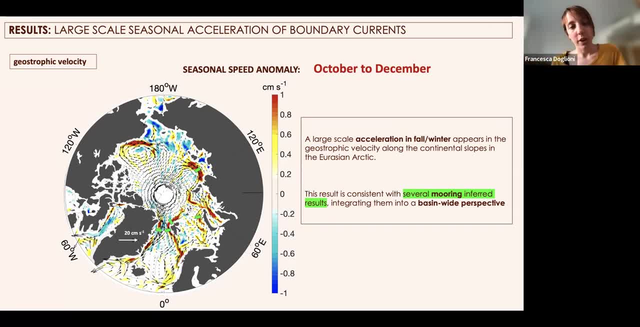 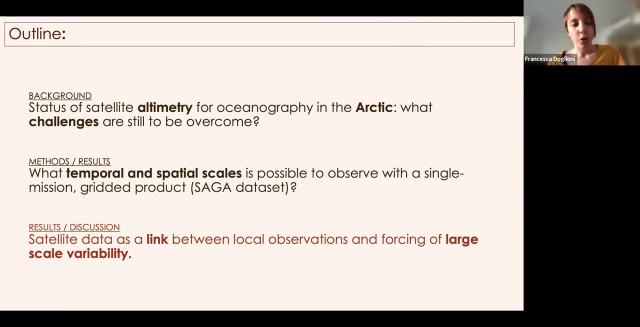 to study boundary currents from a large scale perspective and to integrate several Mooring-based or in situ-based results. And so then we directly go into my third question, which is: can we take advantage of altimetry to understand better the forcing of this large scale? 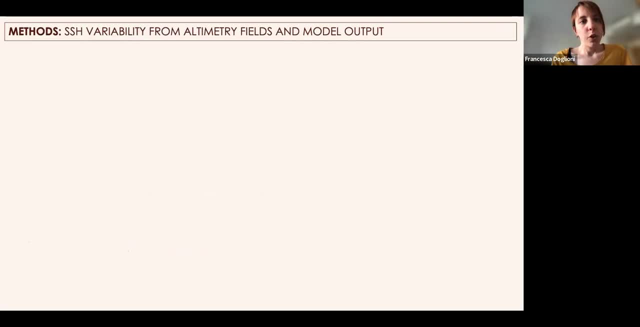 variability. And so to do this, I want to start from a very basic concept of sea surface height and geostrophic currents. So what happens is that the horizontal gradients of sea surface height are related to the strength of geostrophic currents, And as this slope increases, then the geostrophic currents. 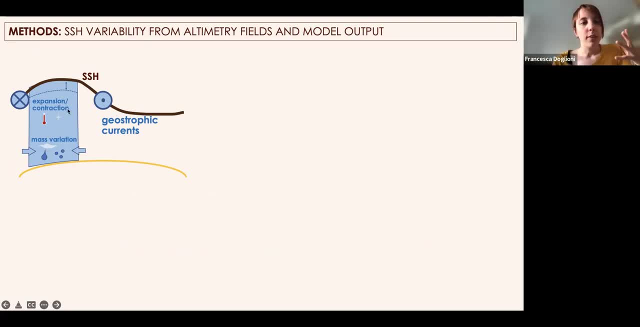 accelerate, But then the variability of the sea surface height. it can be related to, as Ichiro was saying, to steric component, which means expansion or contraction of the water column, or to mass variation, And in this case I will mostly focus. 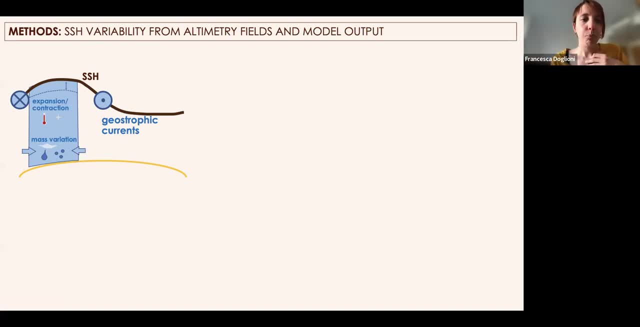 on convergence or divergence of water masses And at this point my question is sorry: what is the nature of the sea surface height variability that contributes to this variability in the slope currents at the seasonal time scale that I've seen before? And to do this I used, as I said, 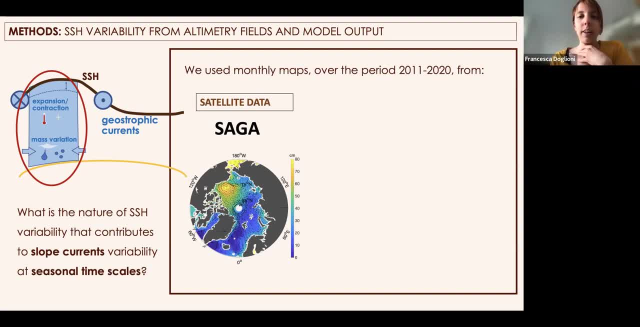 the data from our satellite data set, SAGA, and data from a model, the finite element social model, FASOM, which is a model with high skill in the Arctic, And I used in particular a historical run forced by atmospheric analysis from the GRA55.. 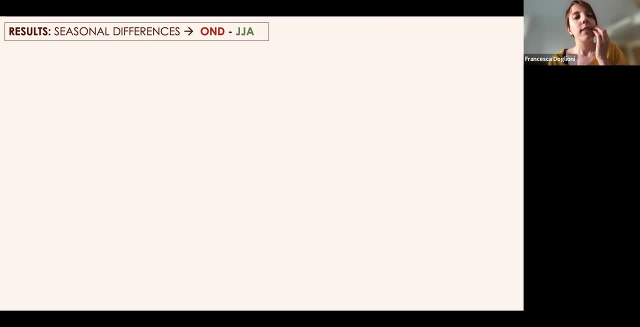 And first thing first, I looked into seasonal differences, differences of sea surface sites, So seasonal differences between winter, early winter period and summer period, And from satellite data we can see that difference in sea surface site between between these two seasons has two main points that I would like to mention. 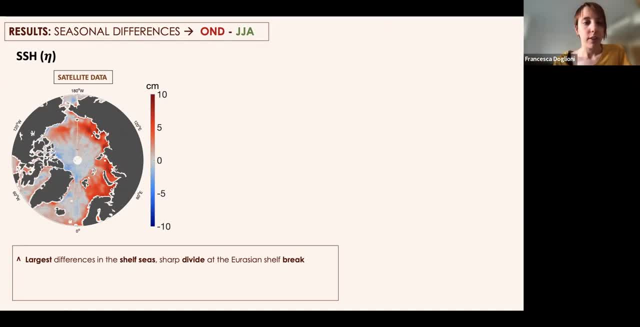 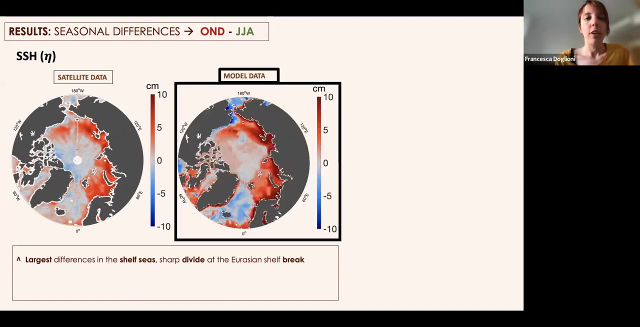 So the largest differences are in the shelf seas And there is also a divide between the shelf regions and the and the and the deep basin, in a sense that the oscillation is in antiphase between these two regions. And so what? what can we see from the model? We can 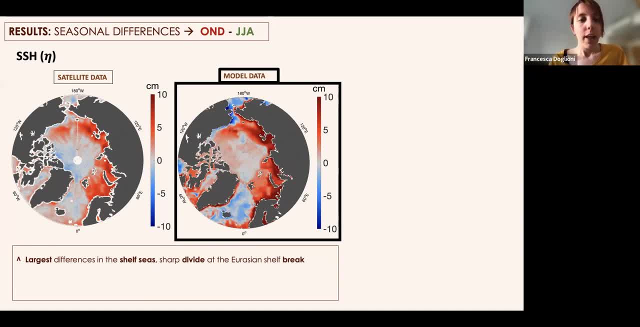 see a very similar pattern. Actually, they agree quite well And, moreover, I can use this model data to further separate the steric differences, seasonal differences, from the mass seasonal differences. So I will show something similar, but just for the, for the variability in the seas of the site due to temperature and salt change. 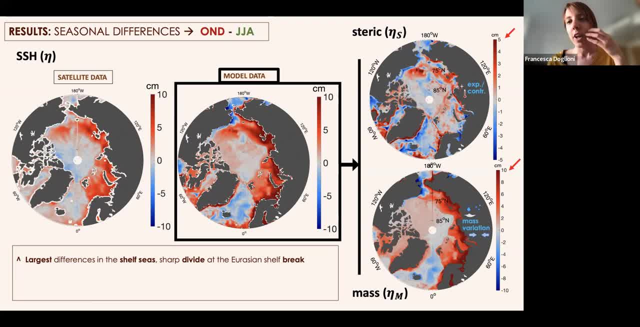 versus mass change. And what happens is, especially if you have a look at the data, you can see that the sea surface has different variances in terms of at the order of magnitude of these changes. you see that the changes in steric height are much weaker and patchy. somehow They are related to very local processes such as river. 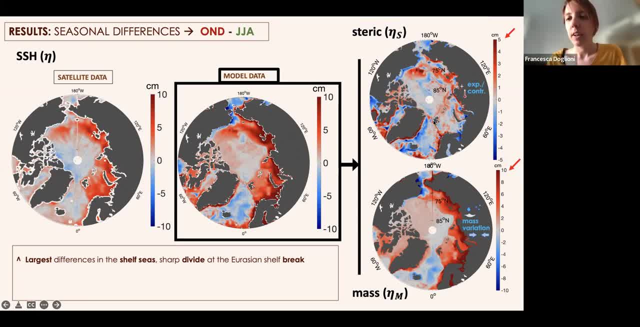 water plume in this case, and Atlantic water flowing along the break or the buffer gyre, as we were hearing from Ichiro- Whereas the mass variability shows a much more consistent large scale behaviour and also reflects this dipole between the shelf region and the deep. 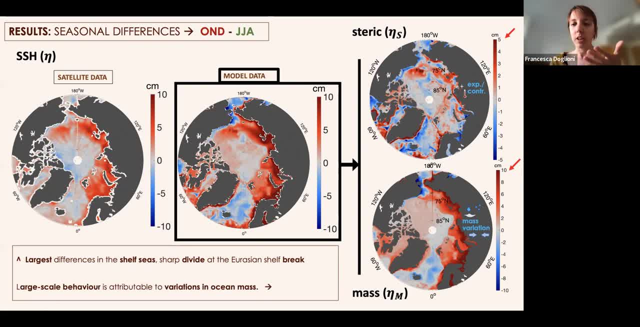 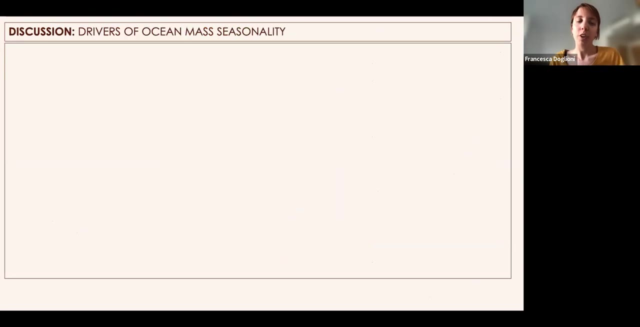 regions. So, actually being interested in what is the variability that modulate this gradient, the sea surface height horizontal gradient between the shelf and the deep regions, I focus on the mass variability, And so up to this point, we have seen some results, and what is now is rather some questions that are still in progress. 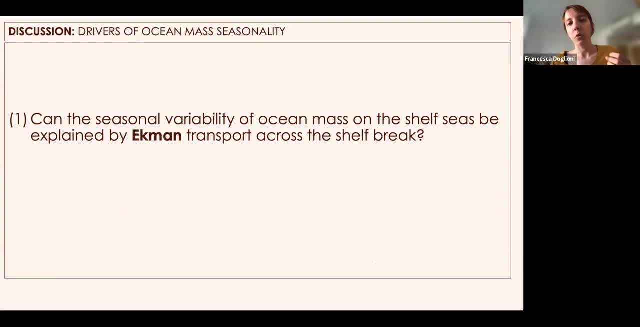 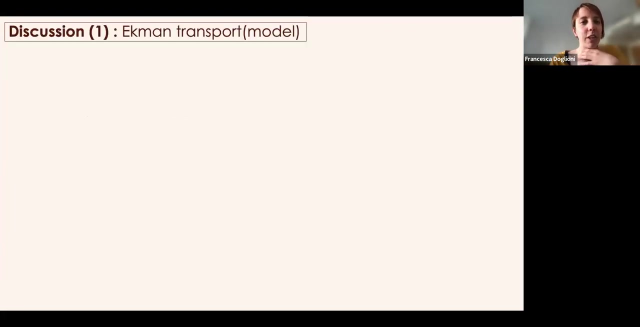 And one of them is: can this seasonal variability of the ocean mass be explained by equine transport in the Ekman changes? These are actually different than the ones you would see in the I Google or the, let's say, the actual kalian's. 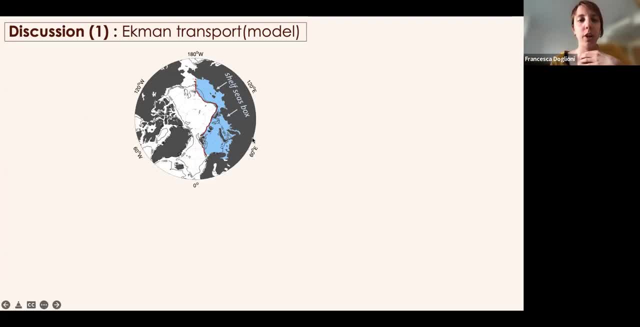 data, and that's where the difference between these two equations is. me, The change is kind of relative to the distance between the deep basin and the shelf, And the second question is: why are these large oscillations so confined to the shelf seas? And so I will give some ideas, and then I hope that these questions can also spark some discussion. 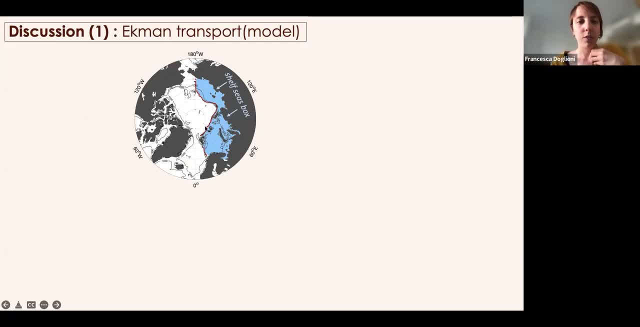 So, firstly, regarding the question on the Ekman transport, what I did is to compute the Ekman transport across this um, this transect into onto the shelf seas, uh, and, and compare it to the variability, uh, to the seasonal cycle in in the ocean mass. and so this is how i calculated the 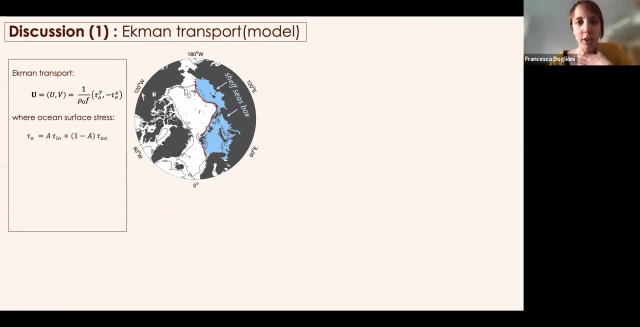 ekman transport, if someone um would like some details, and so i looked at the climatologies. of course, i'm always talking about model data of ocean mass, in this case average of the, the whole shelf seas box and the time integrated ekman transport, and and what results is that um? 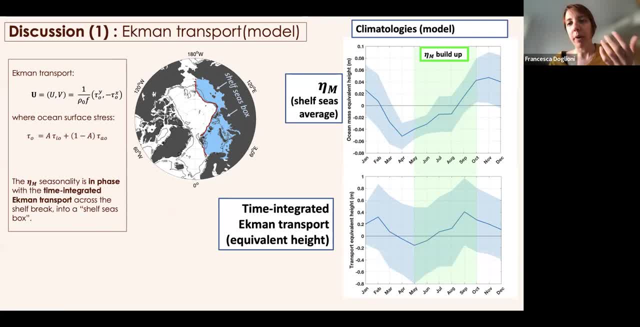 both these climatologies show a buildup of mass on the shelf in in the summer period and early winter, so they are in phase. we can see some relation, but um, at the same time we see there is a big difference in the uh, in the order of magnitude. so the 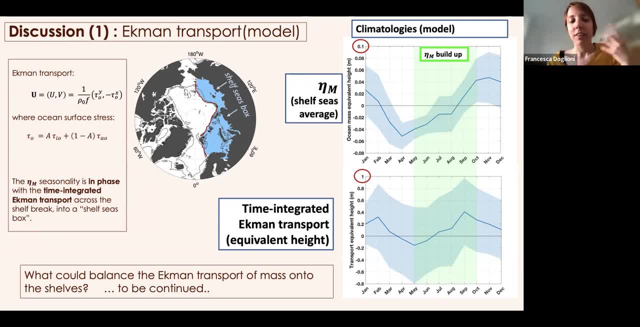 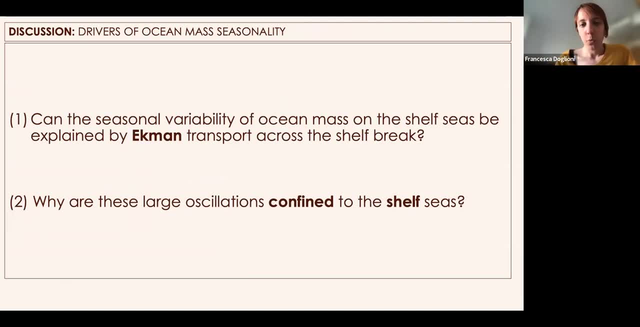 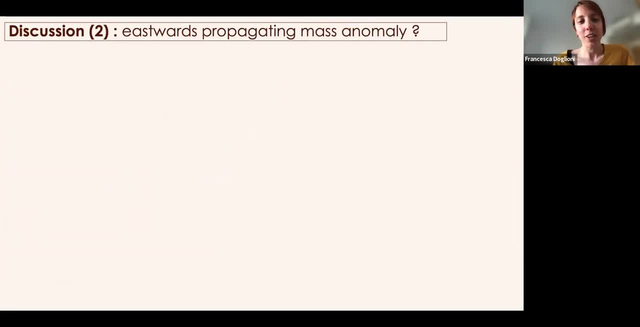 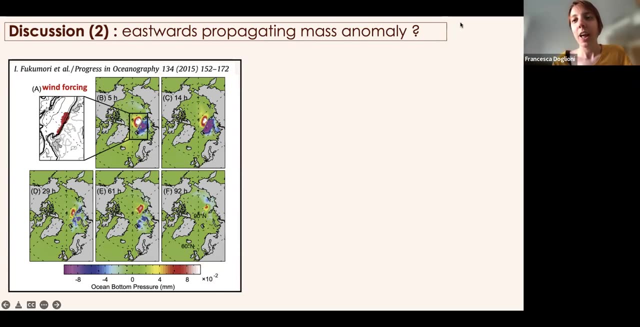 um here. as i said, i was saying to ichiro that i was happy that he is here because i put another figure from the same paper that he was mentioning actually, um, where they in this study day, uh for uh they, they applied some anomalous wind forcing along the shelf northeast of svalbard and they 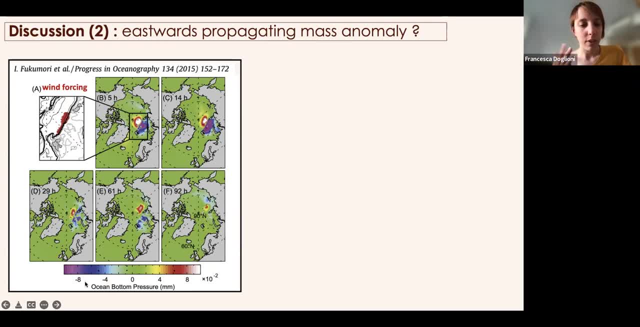 observed how the ocean bottom pressure, which is uh the same as ocean mass, basically uh how it evolves. so there is, there are two mass anomalies that uh develop across the shelf, and then they travel along the shelf. then, in this case, the wind forcing stops um. so they applied some anomalous wind forcing. 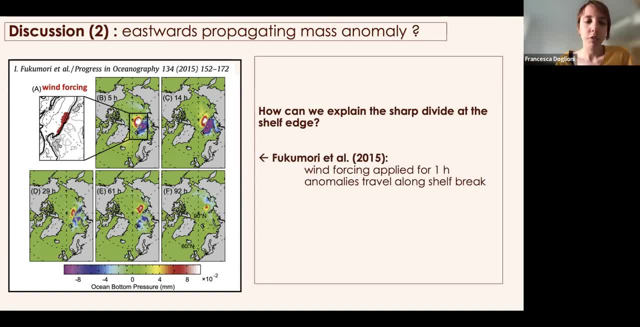 for one one hour, and then the wind stop, forcing stops, and so the two anomalies can sell each other again. but then my question is: what happens if, instead, this wind, anomalous wind forcing, is seasonal and, um, could it actually, uh, so our seasonality on the shelf? could it be related to? 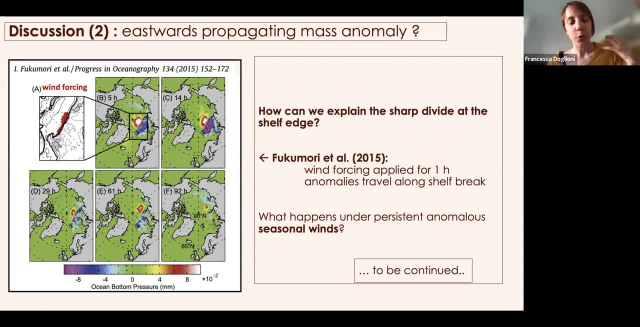 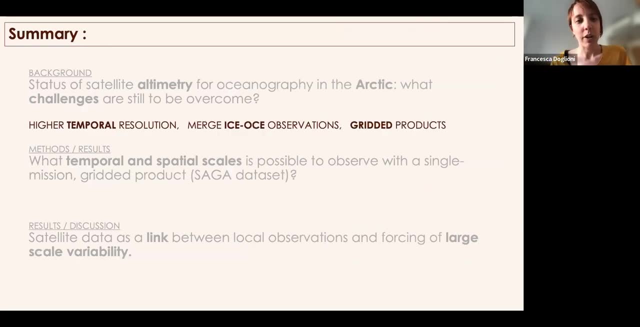 similar process, but this is also- um, i haven't done further, um, i haven't had the opportunity to do that, had further results on this so far. um, so, uh, coming to summarize, uh, my my talk. the first question was, uh, what was the status of altimetry in the arctic and what are the challenges? so, from my 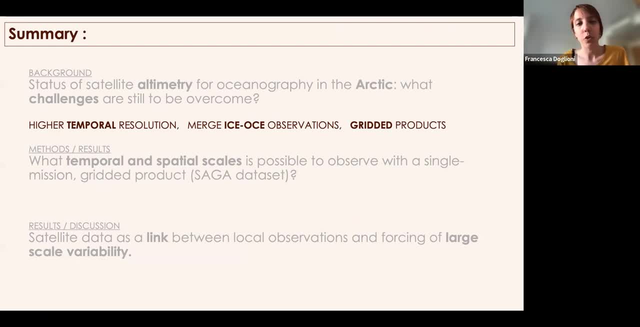 point of view, especially, there is a need of higher temporary resolution and uh, to have merged uh observations from all open ocean areas and ice covered areas, And then that this data are actually graded for climate studies. And then, secondly, we have seen that even with a product, 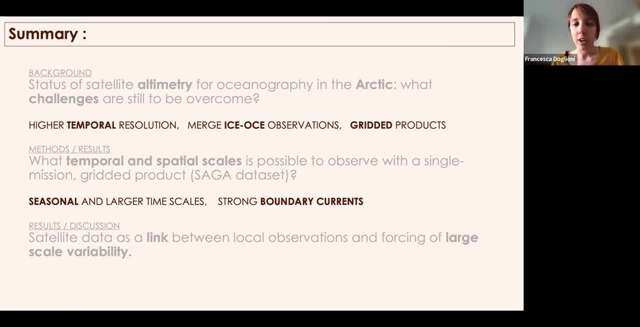 using a single mission, you can resolve seasonal and larger timescales. especially, you can study boundary currents. And then, finally, talking about the boundary current seasonality or sea level seasonality, we see that in the shelf there are seasonal mass oscillations. 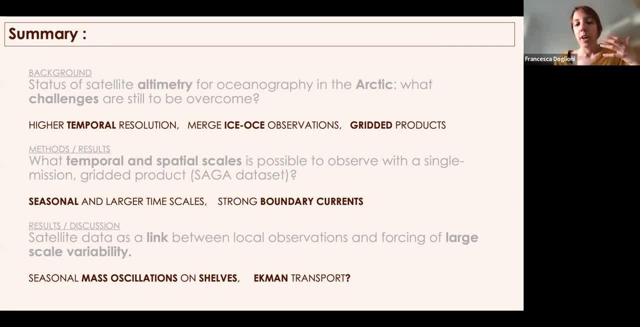 and that possibly are related to Ekman transport across the shelf, break onto the shelf And yeah, that's it from my side And, please, I'm happy to have a further discussion on this and answer. try to answer questions Excellent. Thank you so much, Francesca. 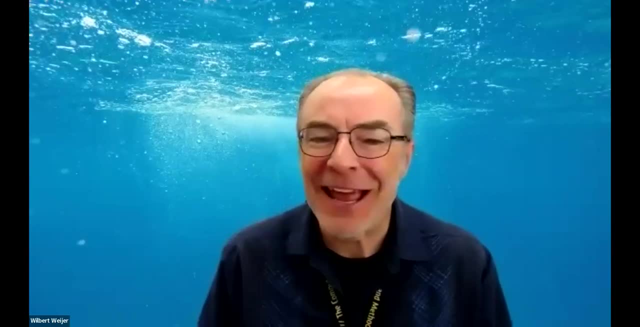 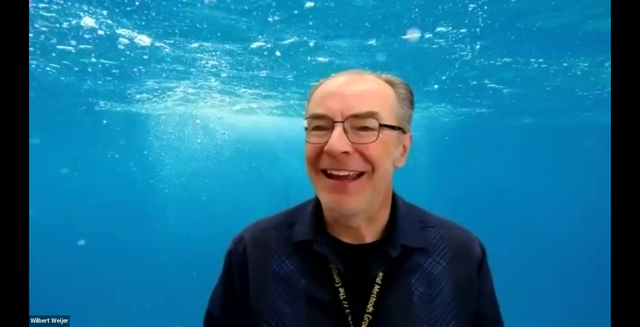 It was extremely interesting presentation and very nicely complementary to what Ishiro shared. Yeah, I was really happy. That's perfect. Thank you very much. So I already see a couple of hands up And of course, Mike is the first one. 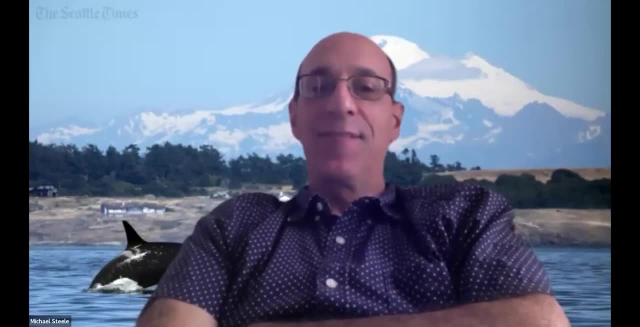 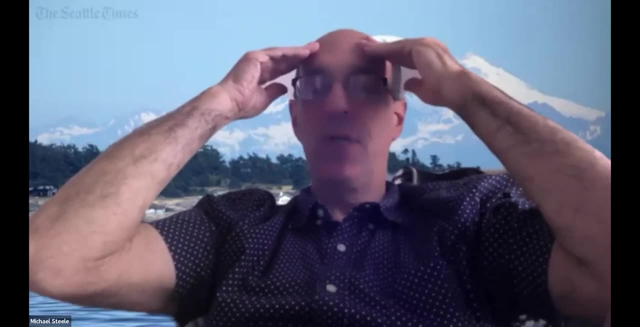 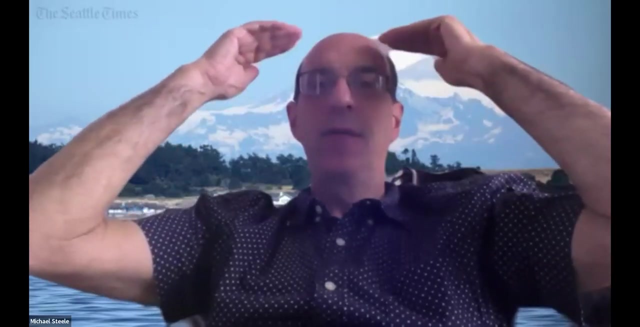 Of course. Well, again, another really really interesting talk, Thank you. So here's my question. I mean, the science was really interesting, but I want to talk about the data set. just ask a question. So there's the Armitage data set and there's your data set. 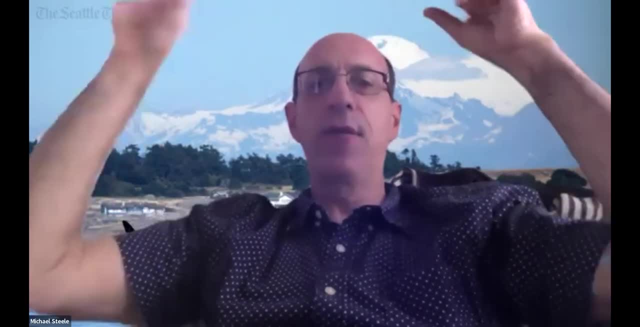 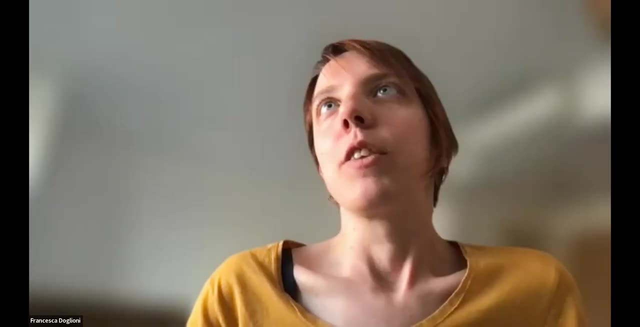 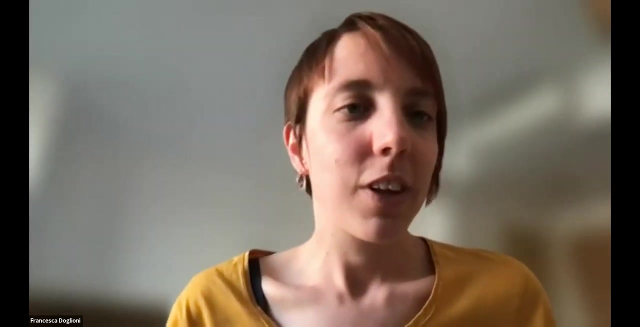 And what do I do if is yours later than his? Like? what do I do if I want, like, a long time series? Yeah, so I think in that case, at this point in time, they are carrying on with the reprocessing of data. 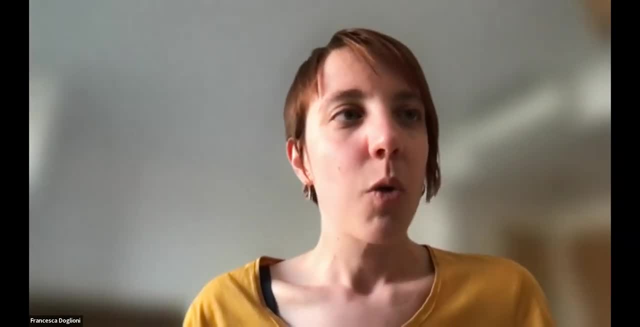 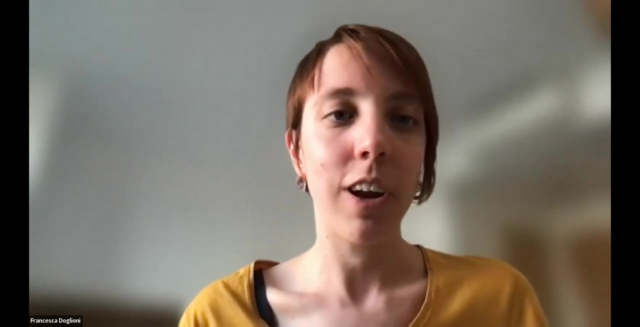 and they have also extended the time series. But what I think, so also in my paper, I am comparing the two data sets And they do correlate well over most of the Arctic, but there are some regions where there is lower correlation or the larger root mean square differences. 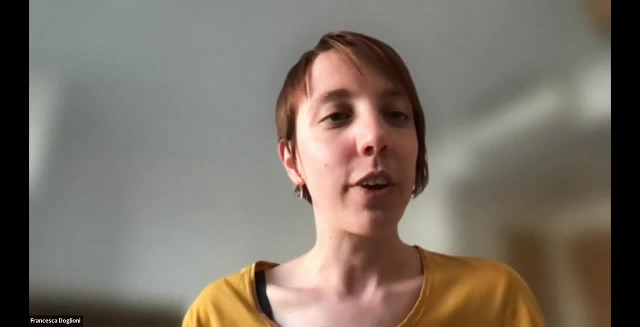 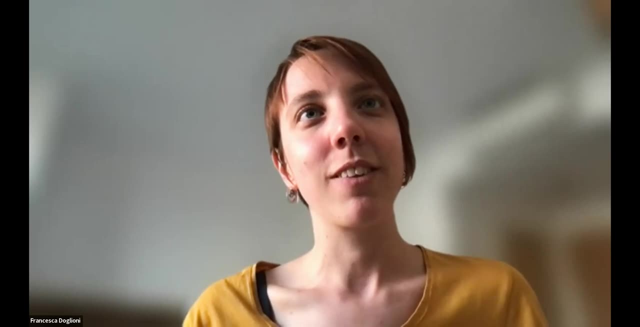 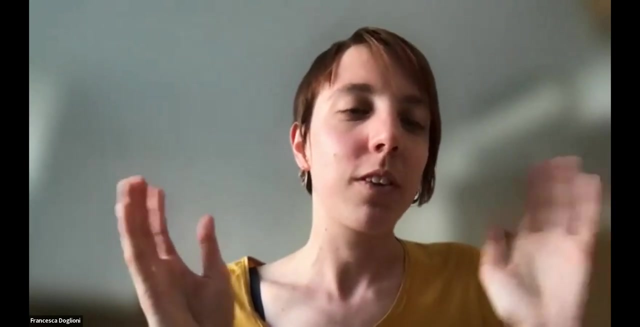 So what my point is? I think at some point also these kind of grid data set will result as sort of as if you were thinking of models: you don't use one model because you have so much uncertainty, And so you'd rather use an ensemble. let's say: 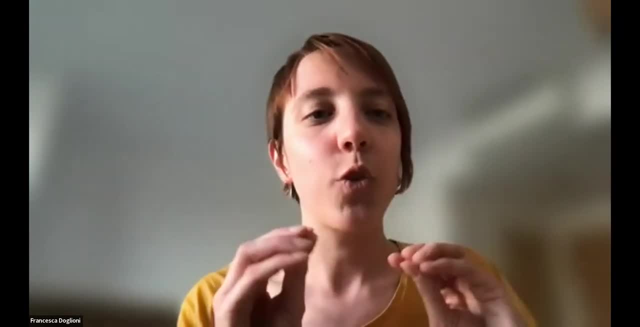 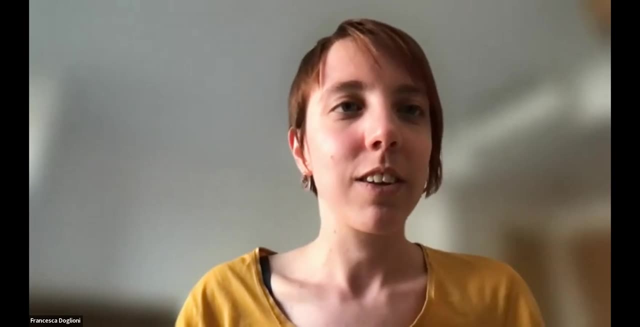 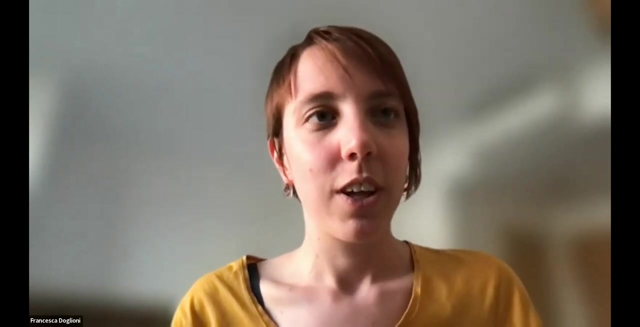 And I think everyone is trying, for instance, different corrections and different, and I think that the idea in the end is that each of these data set can offer you something a bit different. Of course, I think at some point there might be one big institution taking over. 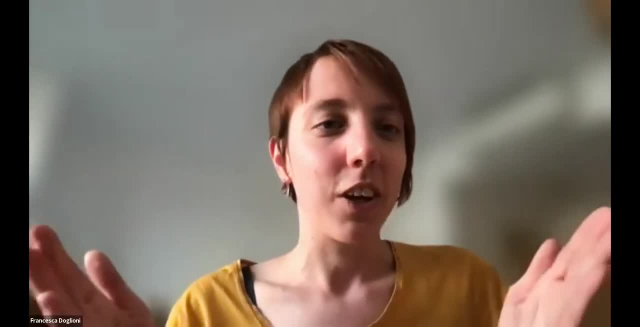 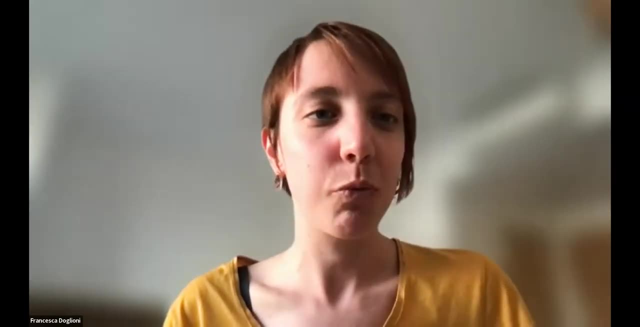 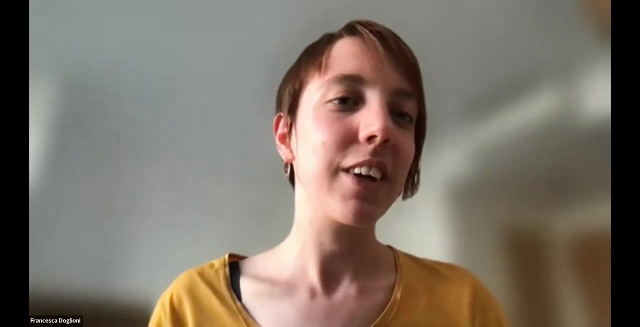 and really opening a team that does this, because otherwise there will always be lots of uncertainty in these kind of products, And I think that we are on the way, but I think we are not there yet. So, yeah, that's my overall answer. 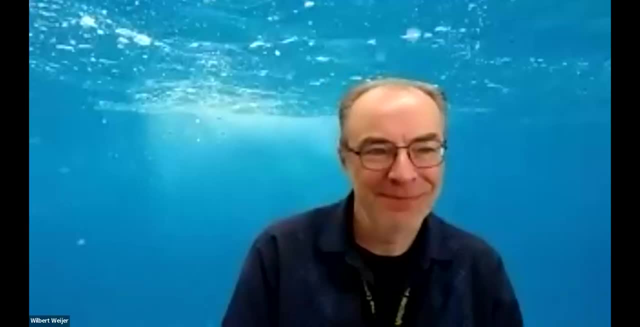 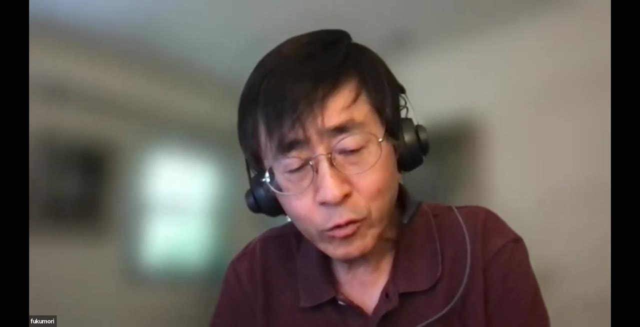 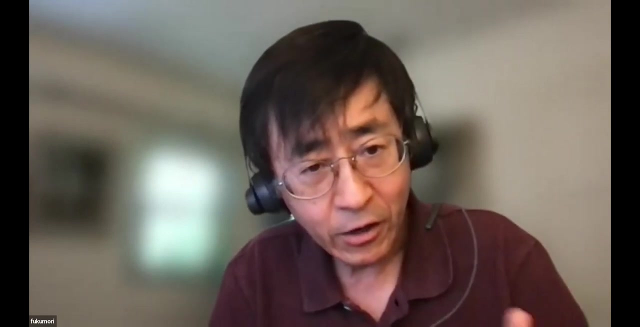 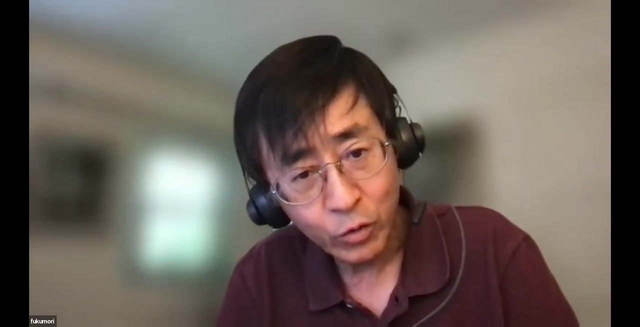 Yeah, Thank you, Shira. Yes, hi, Thank you for a very interesting analysis and data. I have two questions regarding the data and a comment Regarding the data. how much data are there actually goes into a monthly map? How close can you get to the coast? 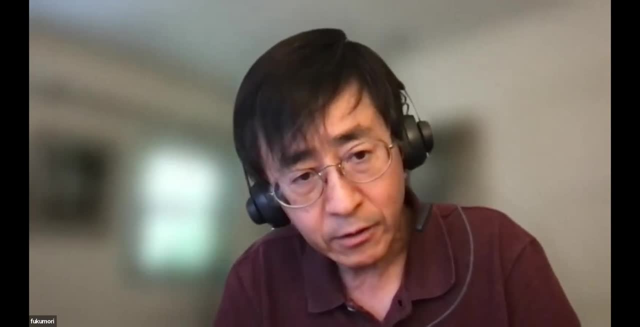 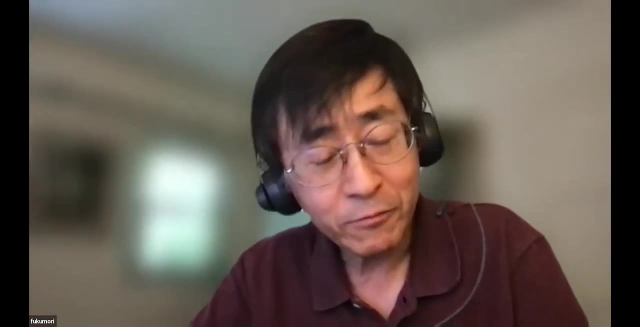 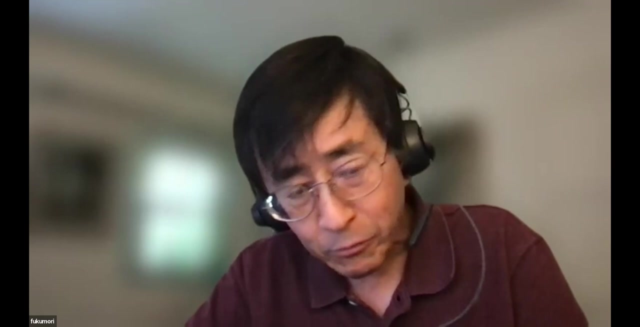 And also is possible aliasing of the kind of barotropic fast motion that was part of my talk. Is that a concern? possibly, if you don't have enough data. And one comment I have at the end is regarding the shelf mass. 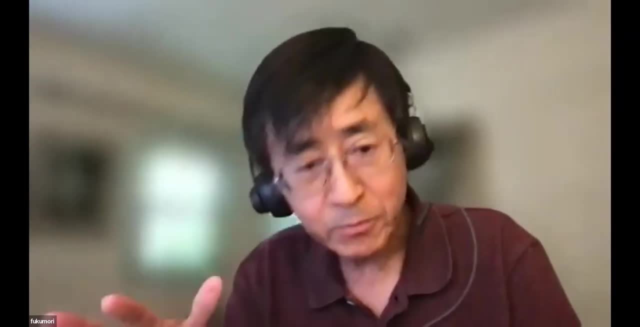 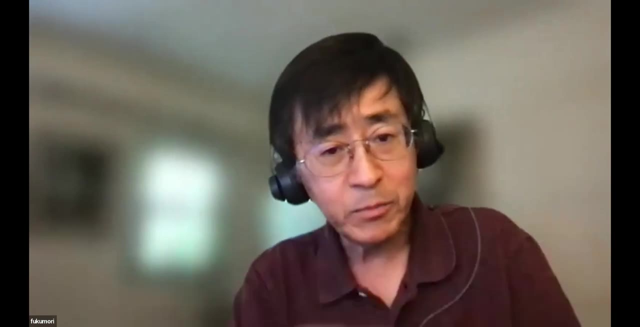 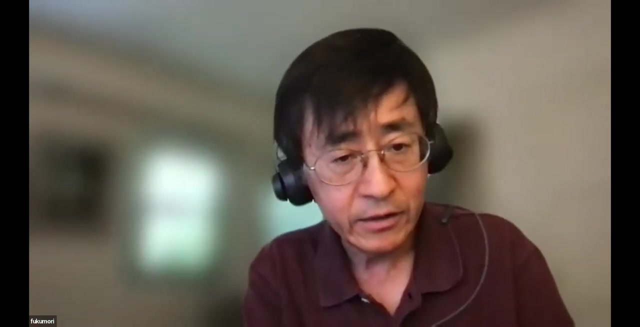 You looked at the Ekman transport. Another possibility might be coastal waves coming in from the North Atlantic, going in and then spilling over into the deep ocean, but still on the shelf, Which will cause a difference between mass on the shelf and in the deep ocean. I wonder whether you've considered that too. So two-part question. I think I will try to answer one at a time and then maybe you can repeat the second one. Yeah, so some data get quite close to the coast. I think rather a limitation is in the Canadian Arctic. 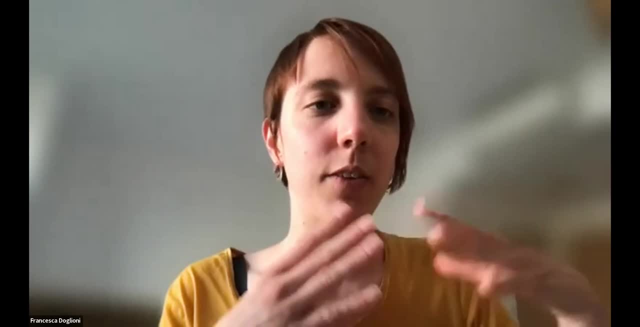 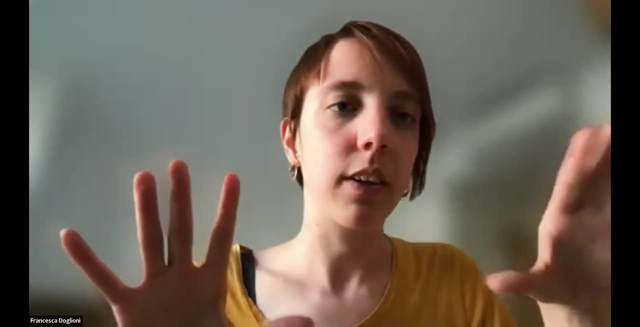 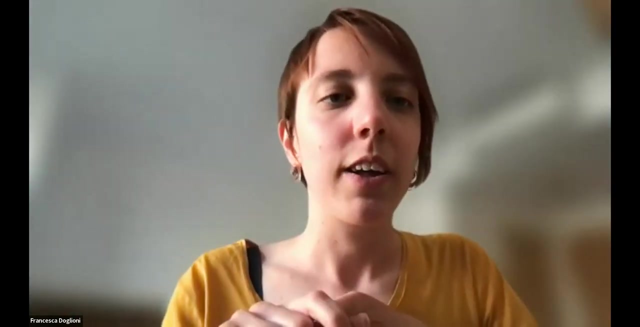 like very packed, And then you don't have much leads, And so in that region you rather have scarcer observations. In my case I also put a mask, a coastal mask, So I just excluded data from 10 kilometers from the coast. 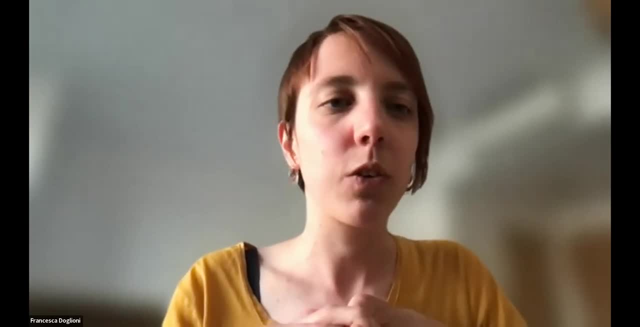 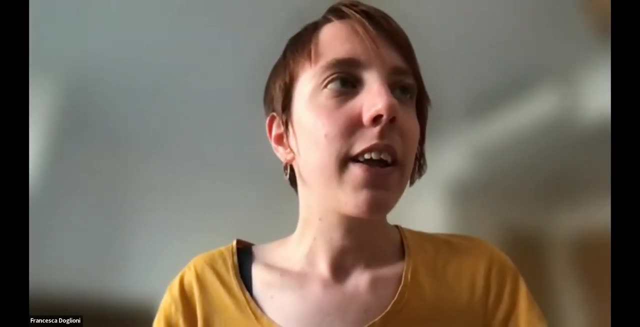 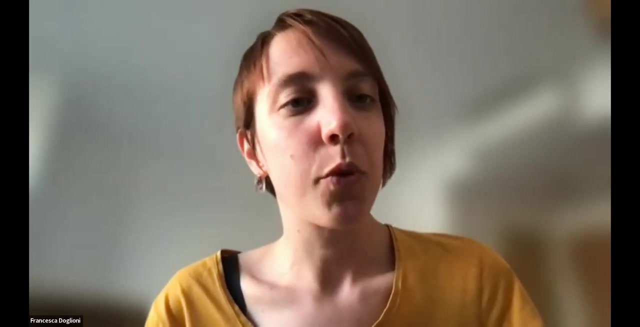 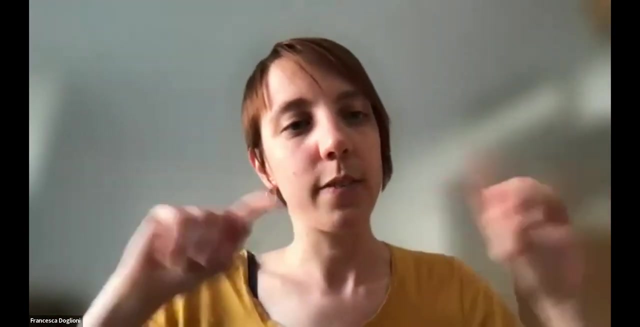 But yeah, I couldn't say exactly how close that goes, But then there were data points even closer And then, as I said, this height, But then there are some very high frequency. variability is really an issue, Because if you have seen some raw altimetry maps in the Arctic, 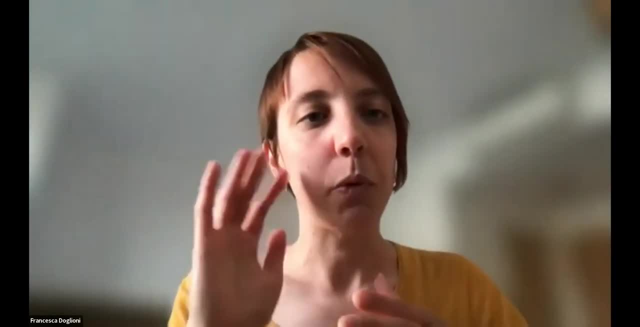 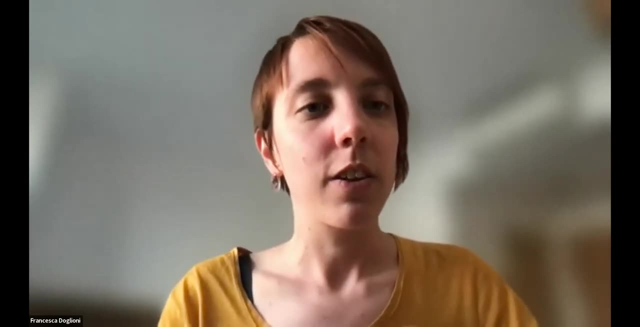 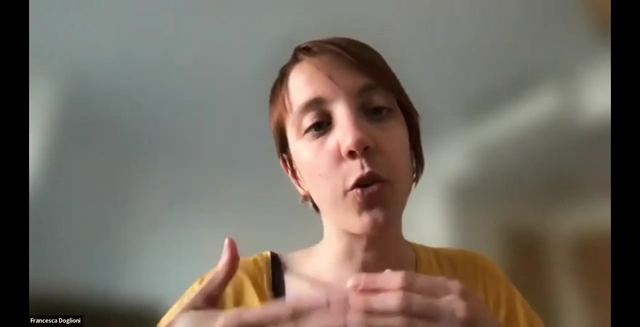 they look very stripy Because there is some past barotropic waves which are not resolved and cannot be really very well corrected. They're difficult to remove. So the two options are Other. So you have to find a good, let's say a model correction. Because that's usually what's done in satellite altimetry that you use a model to, And there is this: one of the corrections that is applied is called dynamic atmospheric correction, which is similar to an inverted barometer, But rather it also contains some very high frequency variability. 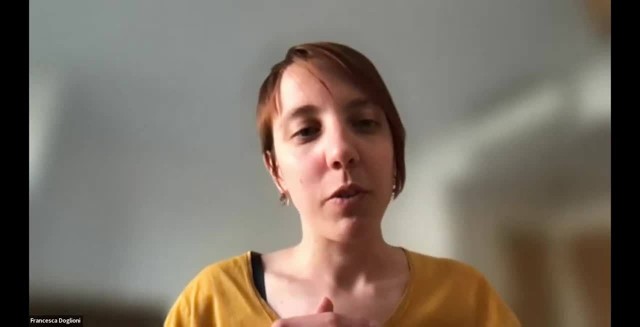 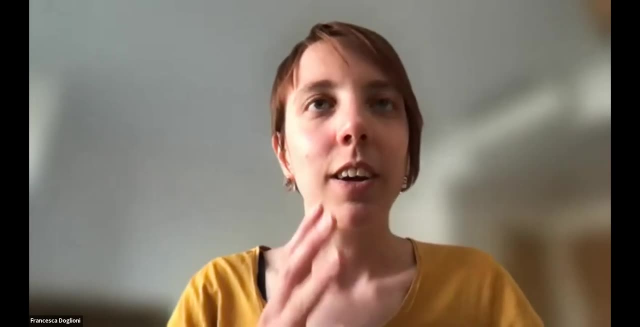 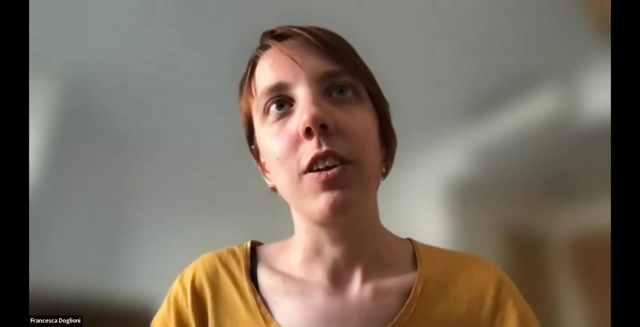 that is not really very well corrected. So you have to find a good, let's say, model correction That contains barotropic waves traveling, But I think in the Arctic this might be still not a very Yeah. I mean the model from which this correction derived. 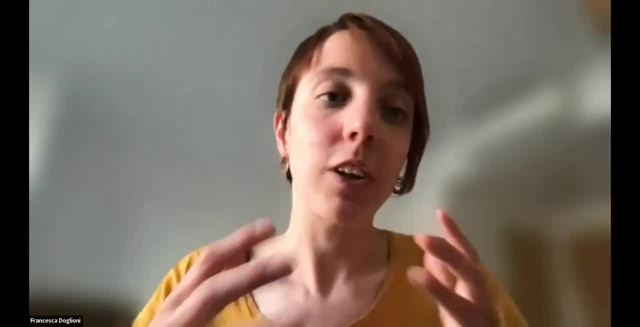 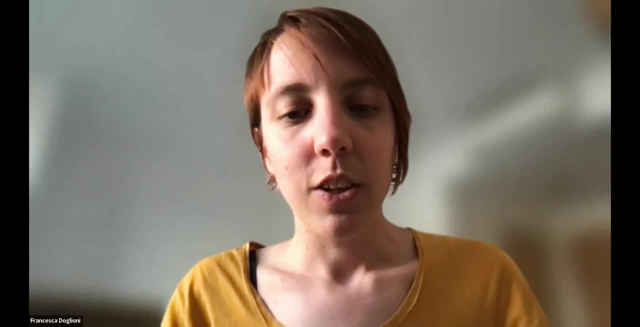 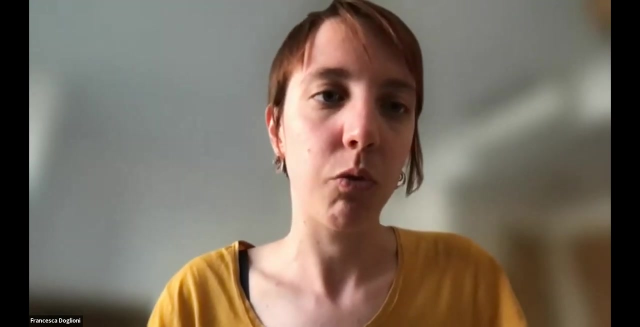 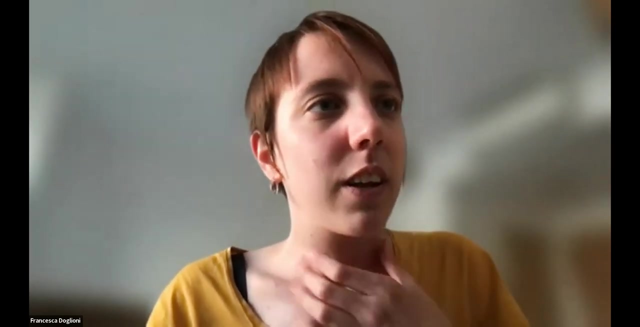 might not be the best. The region might not be the best region where this acts. So there is definitely an issue about removing high frequency variability from the. if you use data at least from one satellite, Yeah, And then I think, your second question, or comment. 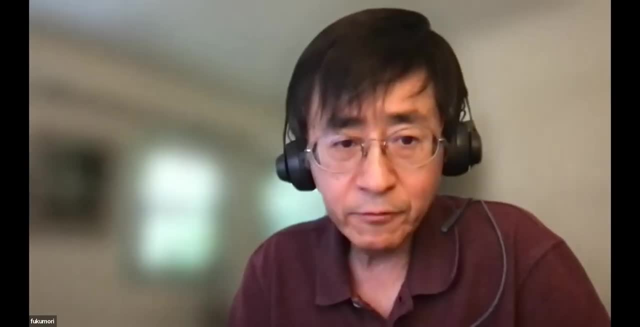 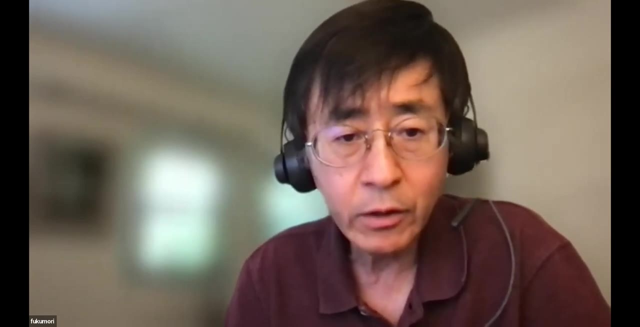 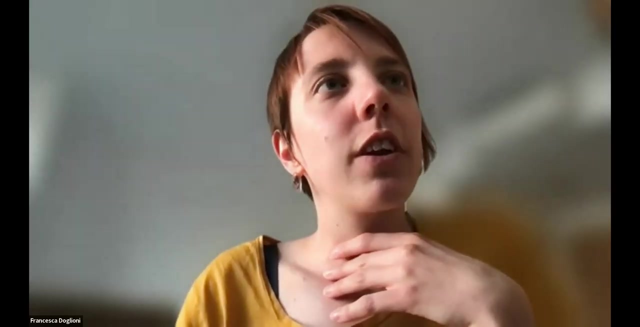 was about waves: Waves from the North Atlantic, for instance, along the coast, which would probably show up in sea level along the coast, but not in the deep ocean. Yeah, So actually so where the idea started, also from your paper. 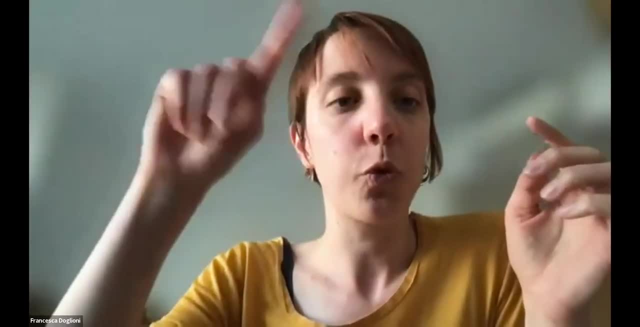 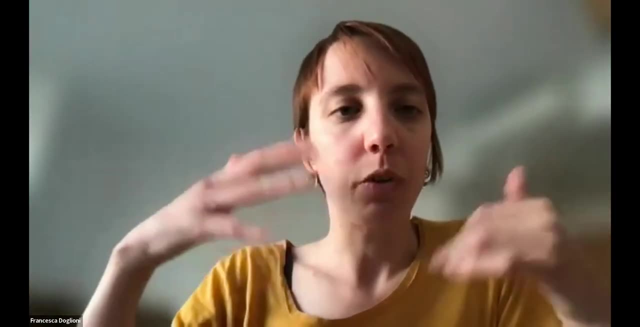 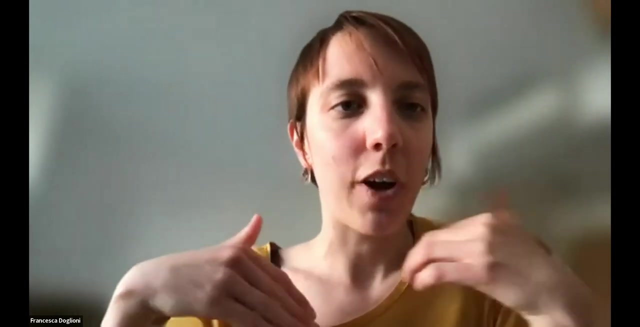 OK, in my case, in the case that I showed, I just showed this wind forcing inside the Arctic, But, if I remember well, you were saying that a lot of variability is due to wind forcing, just like around the Nordic seas or even more south right. 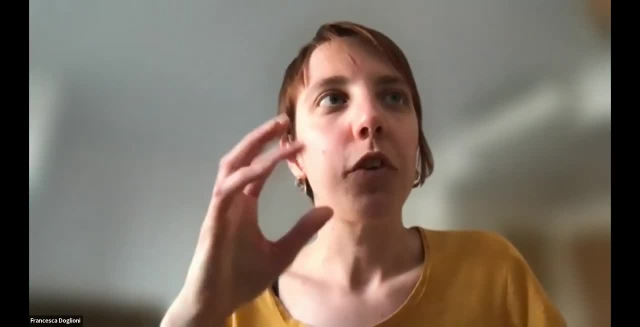 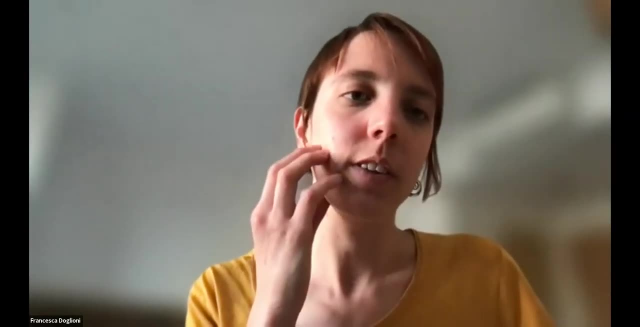 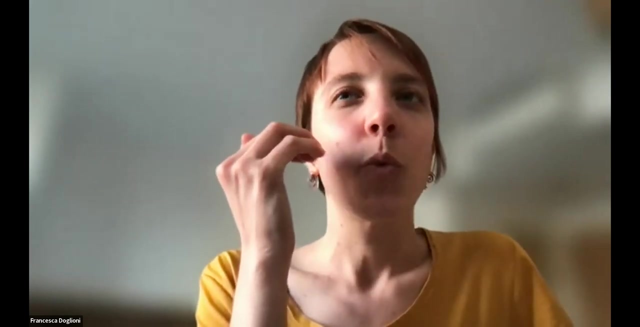 So I still don't capture Very well what could be. But my question is, rather like these waves that you are talking about is, our processes are very fast processes, So what I wonder is whether this can at all have an effect on a seasonal time scale. 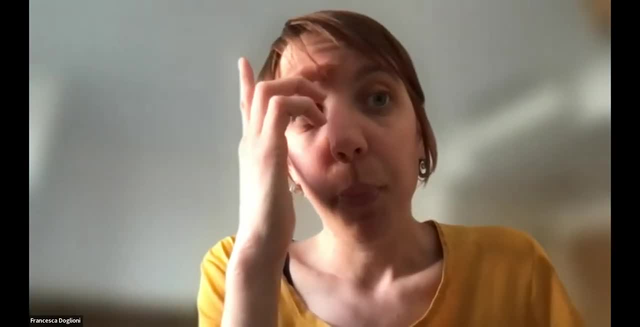 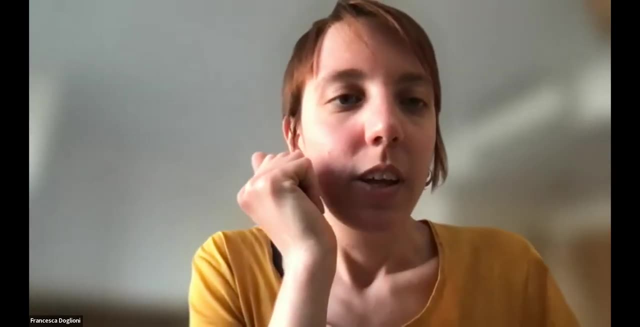 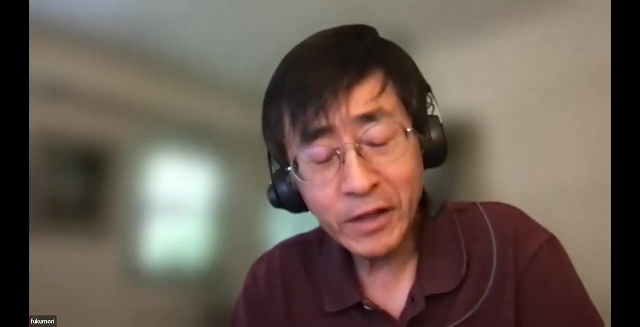 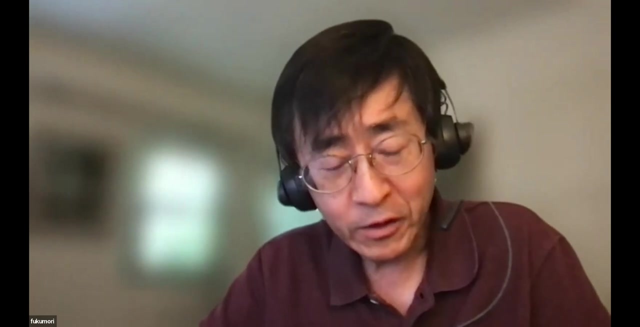 because that's what I'm looking at and how in a way. So Yeah, I don't know if that answers your question. At least in the model that we analyzed, the waves that come from the North Atlantic go into the Arctic on the shelf, then spill over. 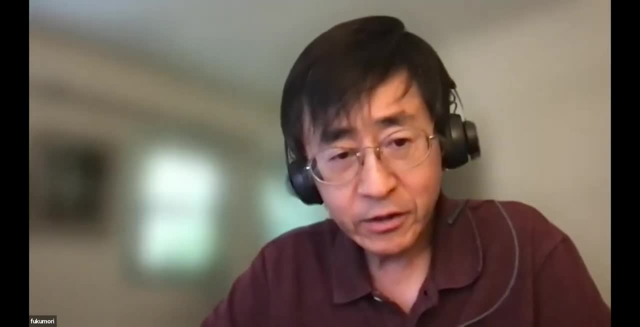 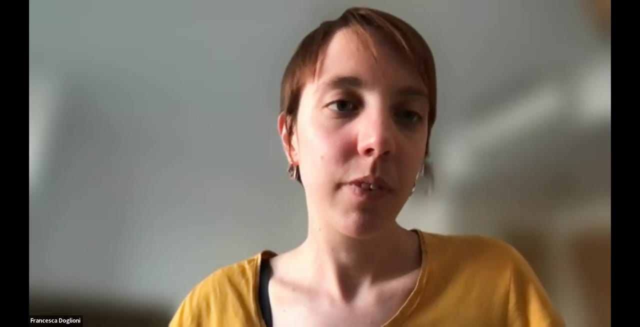 into the deep basin. The part that spills over into the deep basin stays for a long time, but the part on the shelf disappears, just propagates through. So you end up with a mass difference between the shelf and the deep ocean, because the deep ocean part signal just 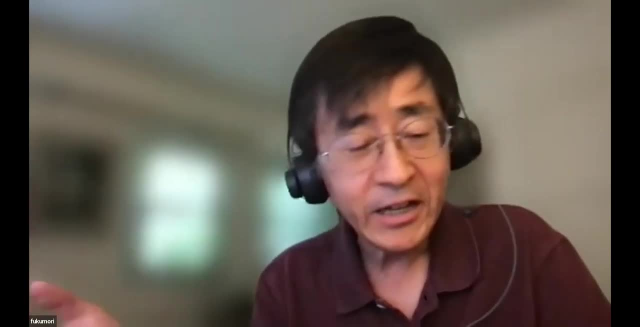 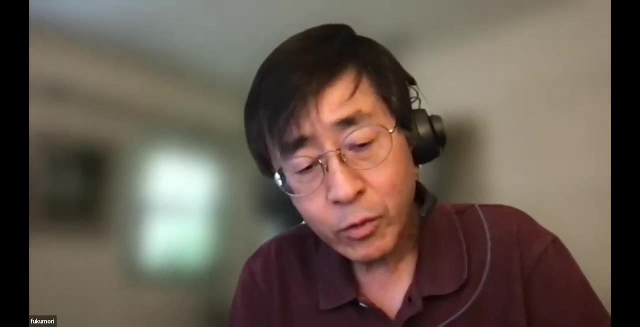 Yeah, Just stays. So it's not that the signal on the shelf stays, It's the. it's a deep ocean, So that signal that stays. So you get this contrast. So I wonder whether you might be seeing some of that effect or not. but I could be wrong. 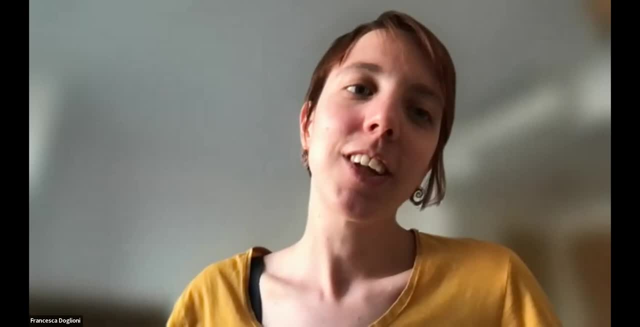 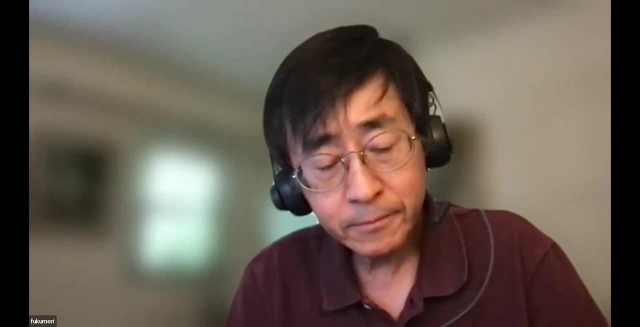 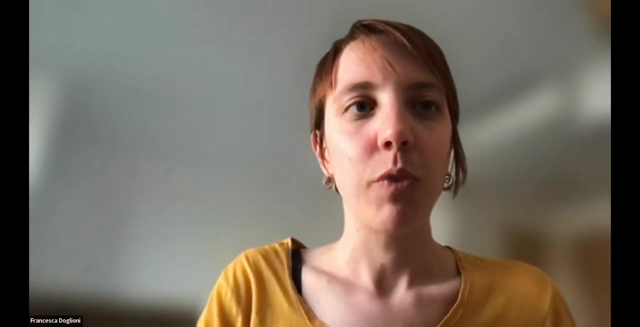 Did you see whether these waves have a seasonality? No, we didn't look at seasonality. No, we haven't, So it might be entirely different. Yeah, what I'm thinking is, of course, if you have this Build up in the, let's say, then in the deep basin, 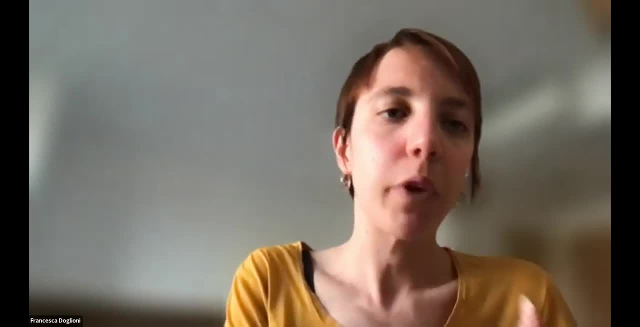 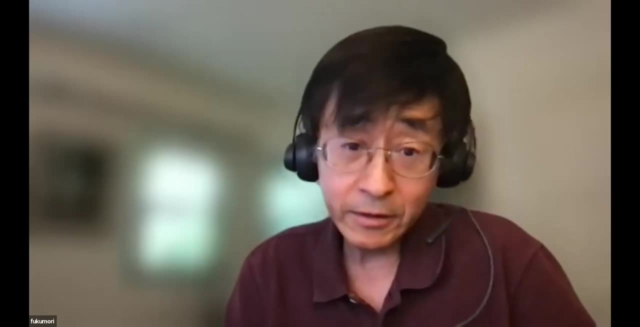 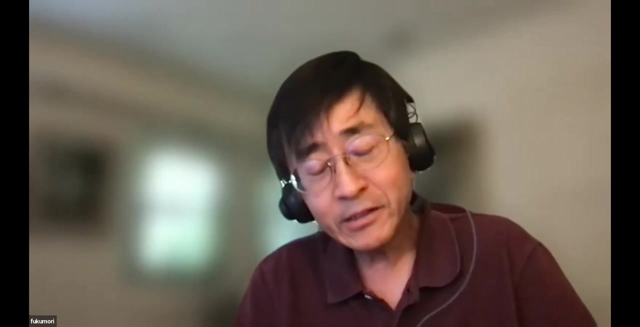 if you have more frequent wave in a certain period in a certain season, that could kind of explain the difference between the two. Possibly there's seasonality in sea ice cover So that could modulate perhaps the wind stress, And seasonality is not something that we looked at. 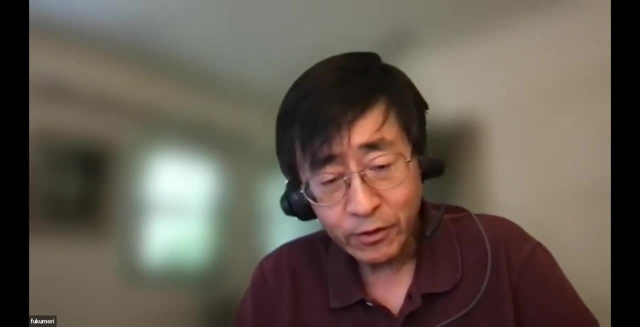 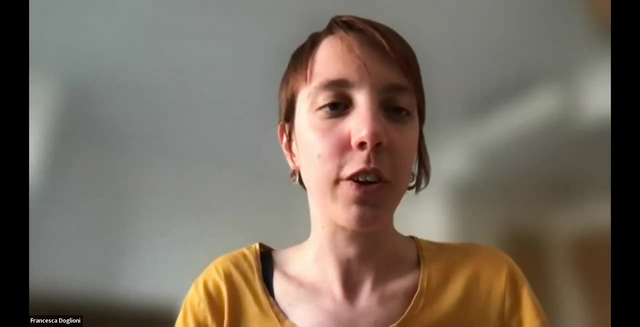 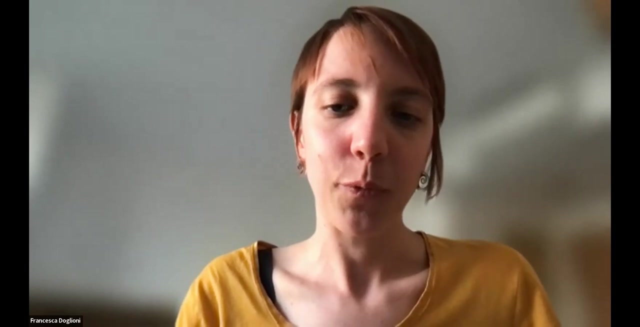 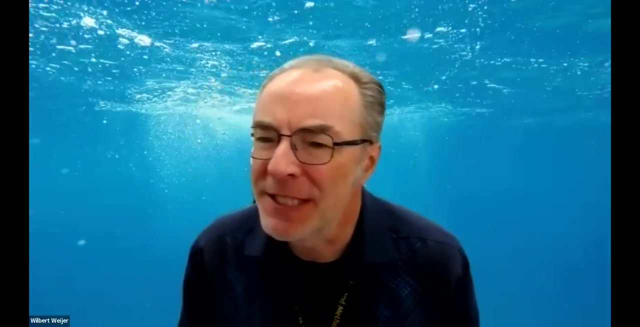 So it might be additional things or different things that go on. Yeah, Difficult to, especially if it's a remote forcing to identify where it can come from. Yeah, Thanks, Thank you. Don't see any more hands raised. Anybody still wants to speak up? 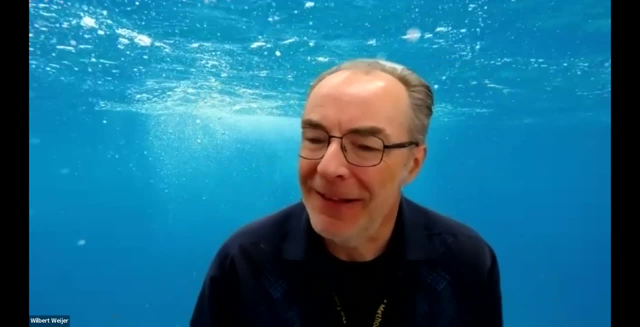 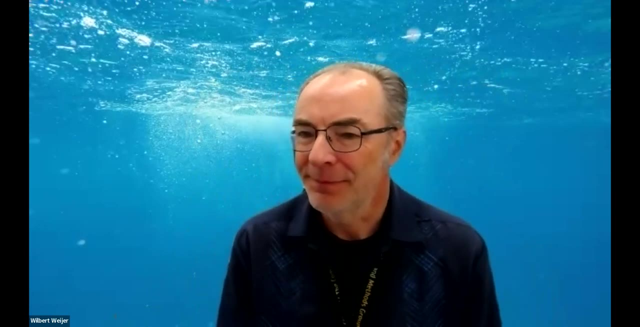 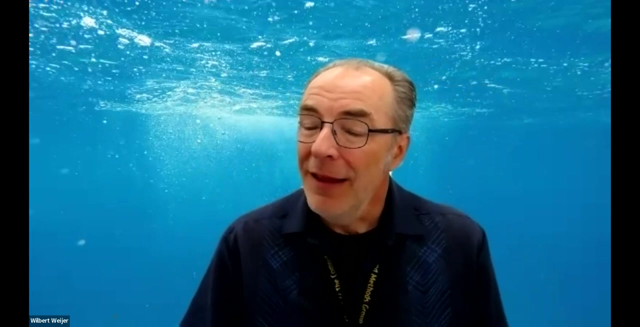 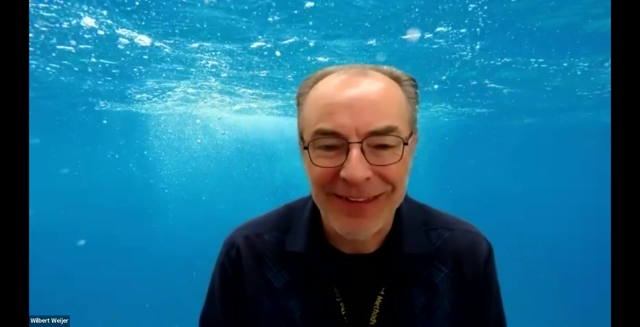 Maybe early career scientists that are on the call. Any questions that you might have for Jessica or Ishiro? All right. If not, it's two minutes before the hour. We can stretch it Or we can just say: well, thank you everybody for joining us. 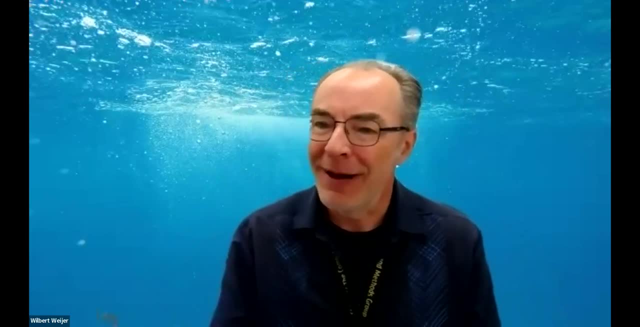 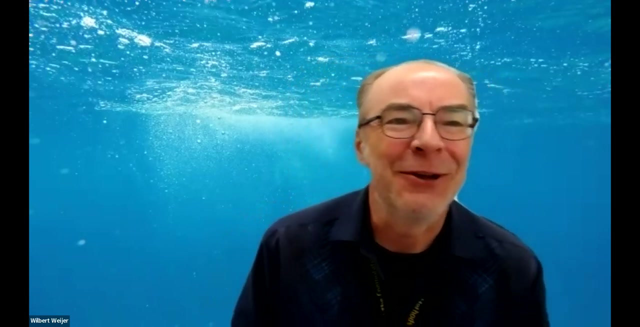 And especially for Jessica and Ishiro for presenting And everybody else for participating in this very interesting discussion, And I really enjoyed this session. It was really, really nice, Mike. Yeah, Are you going to stretch it? Maybe you should unmute yourself. 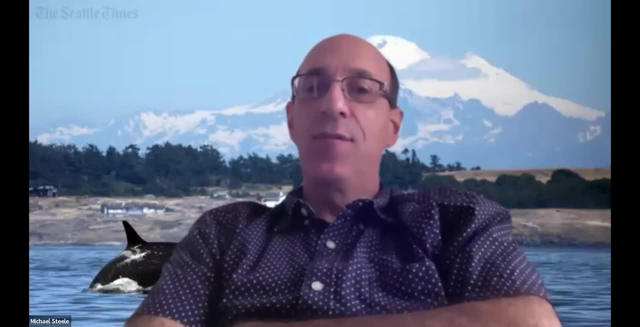 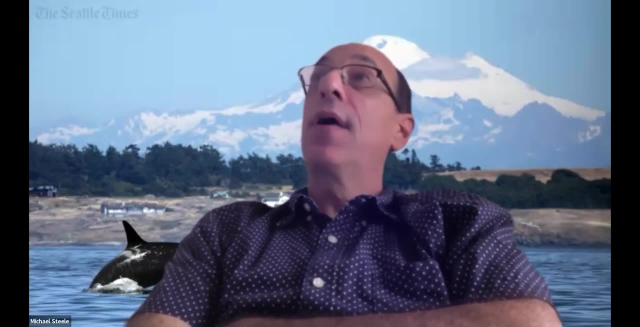 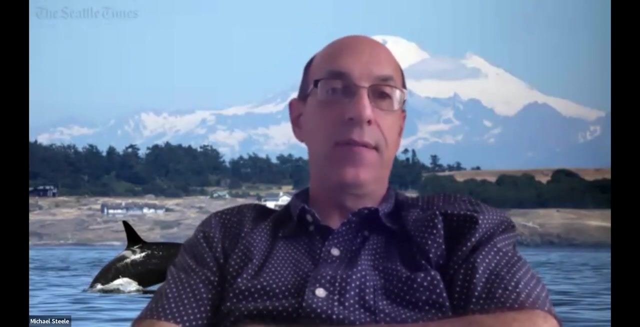 Yeah, sorry. Well, Francesca, I wanted to ask you more about the science then that you were showing, And I want to ask you about off-shelf transport of fresh water. Did you say something about that? Not specifically of fresh water. 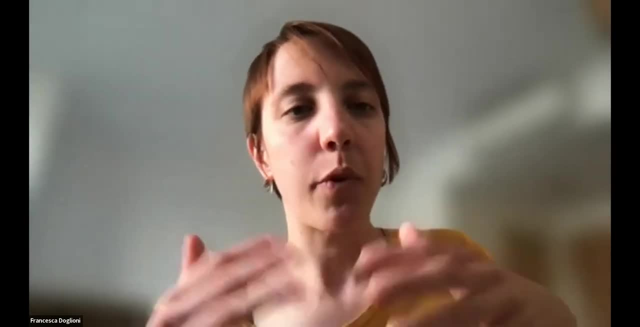 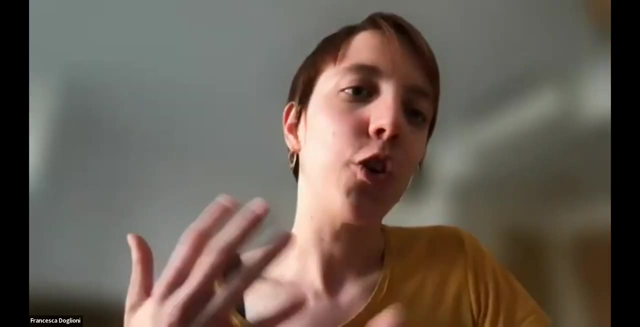 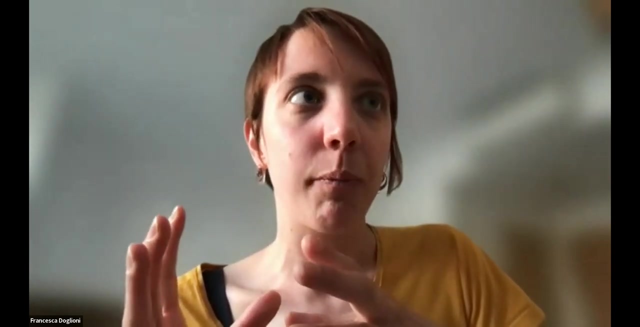 I was meaning Rather. so when I separate the steric component to this mass component, meaning that I compute the steric component and then the residual is basically what I consider as mass component And this I compared, like the variability of this. 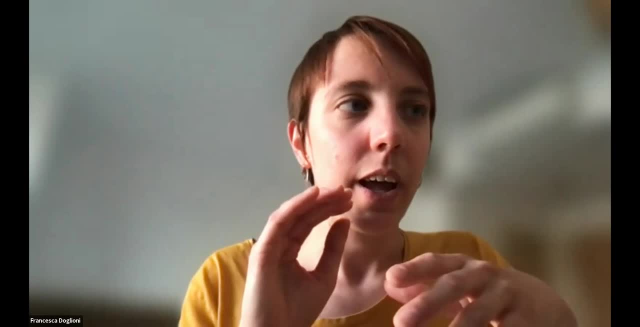 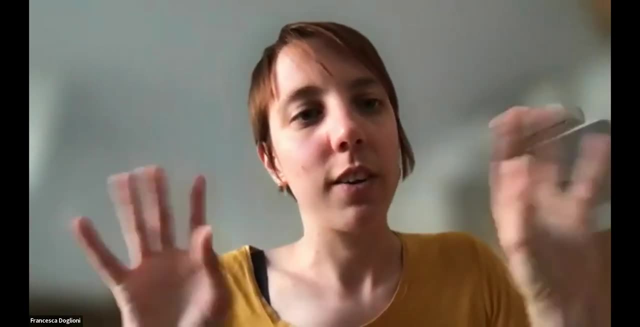 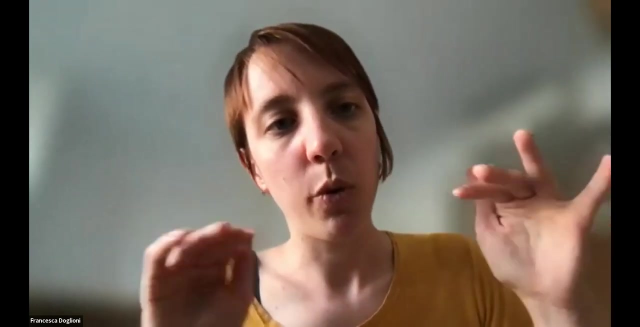 on the shelf. I compared to Ekman transport like time-integrated Ekman transport And that's kind of Like there are separate calculations in the sense that on the one side in the model you have wind flowing, blowing on the ocean or on the ice. 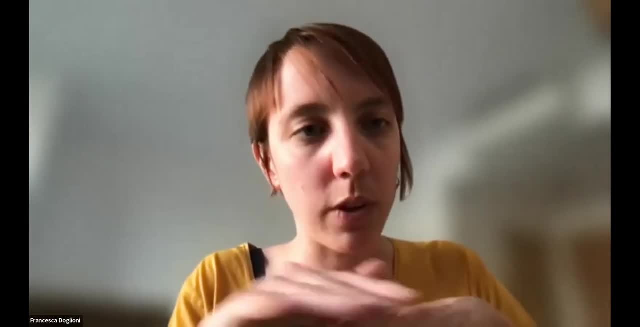 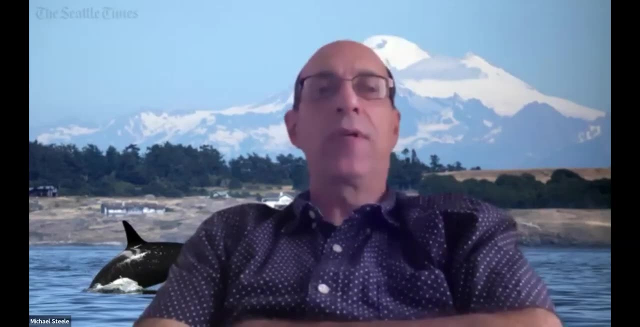 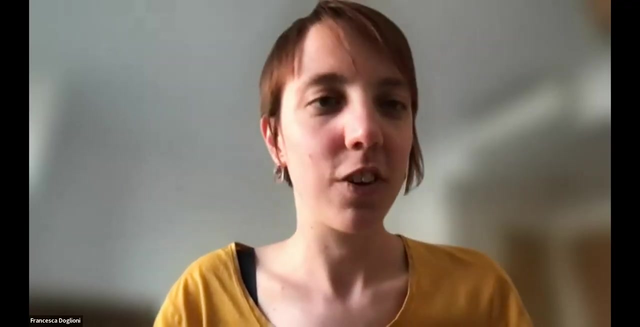 And then from that, like you can actually compute the stress at the surface and the Ekman transport, that yeah, OK, Maybe we can talk offline. I have some interest in that right now. So, OK, Yeah, Maybe I'll send you an email or something.